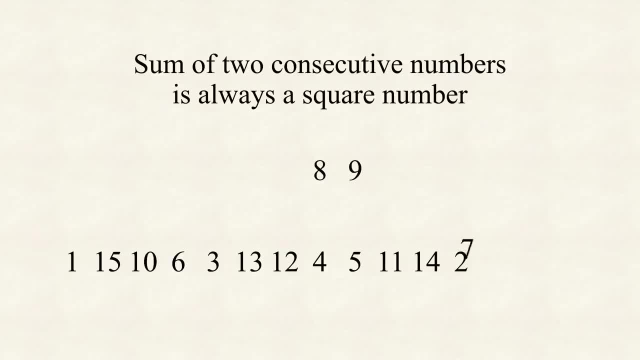 Alright, Oh, so close, but we are missing the 8.. But luckily the 8 fits perfectly in front. One way to illustrate that consecutive numbers have squares as sums is to animate. Take, for instance, the part 12,, 4, 5.. Indeed, 12 plus 4 gives a perfect square. 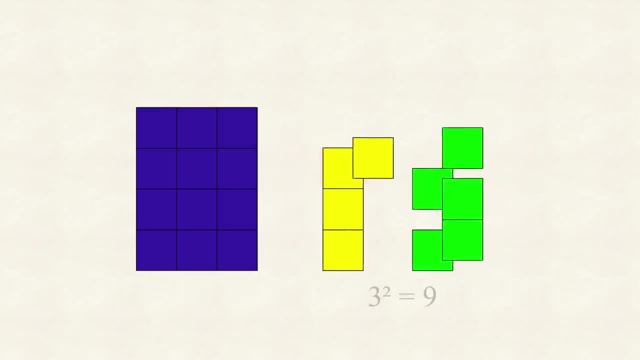 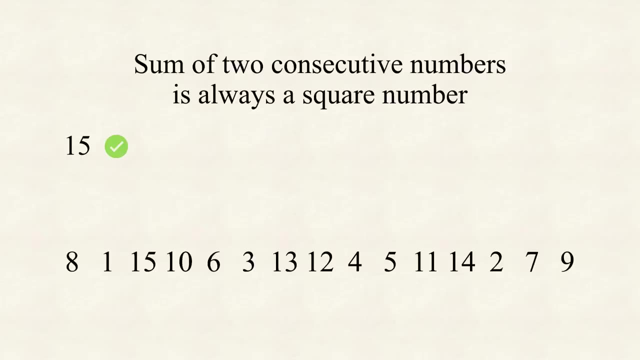 and so does 4 plus 5.. And that's the animation you saw in the beginning. So the answer to our question is yes, We can arrange the numbers from 1 to 15 in that way. The same is true for 1 to 16, simply by adding 16 in the back, giving us a sum of 25.. 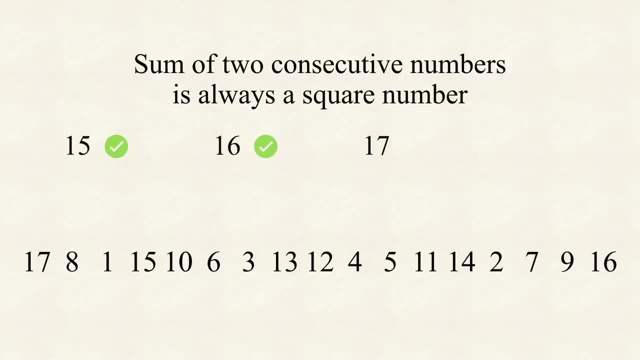 Also, 17 is easy as it fits in front, also with a sum of 25.. However, it turns out that one cannot arrange the numbers from 1 to 18 to have this property. Doesn't matter how hard you try, the problem simply breaks at 18.. 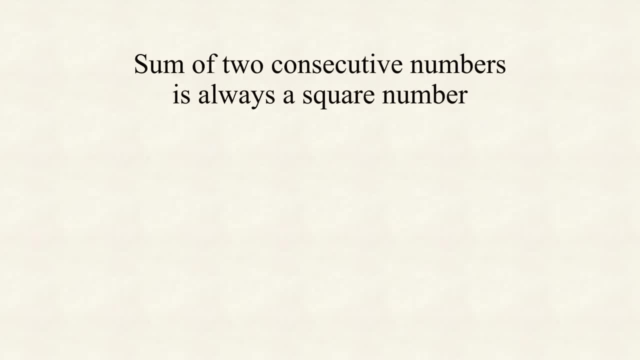 Also, when adding 19 or then 20, the problem has no solution. Only when taking the first 23 numbers, there is again such a solution, And here it is, But for 1 to 24, it is again impossible. Now the great mystery, the problem no one could solve. 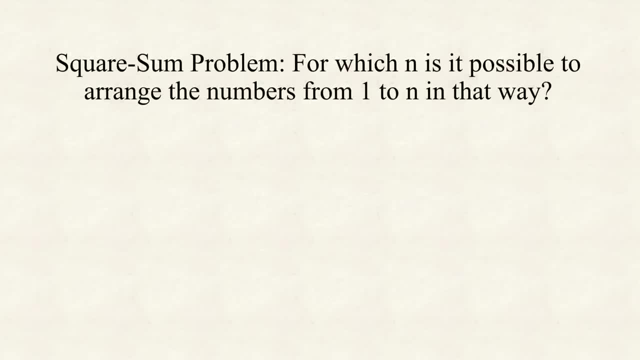 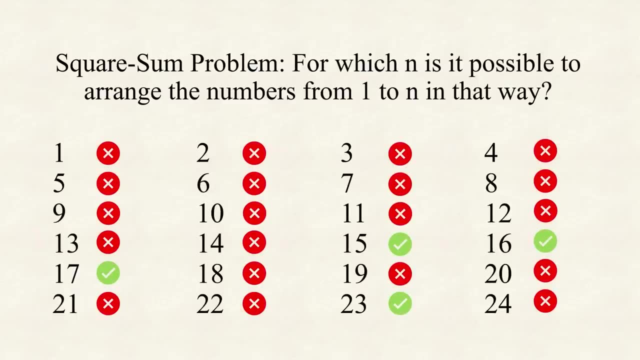 was to find out for which n there exists such a sequence of the numbers from 1 to n, which became known as the square-sum problem. For small numbers, one can figure out by hand which are possible and which are not. As you can see, I picked the number 15 on purpose, as it is the smallest number with this property. 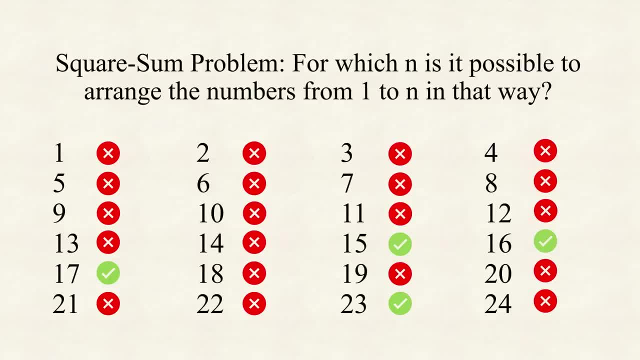 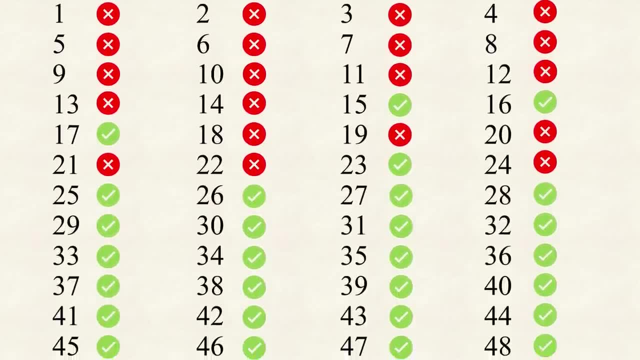 So for some numbers it works, for others it doesn't, But somehow all numbers starting from 25 seem to have this property. So the square-sum problem asks whether such a sequence always exists for every n greater than or equal to 25.. Even though it seems to be true. 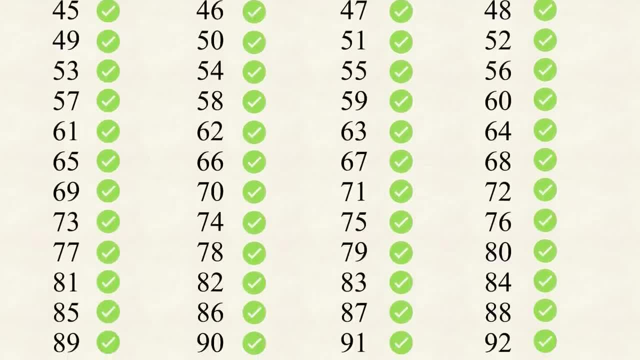 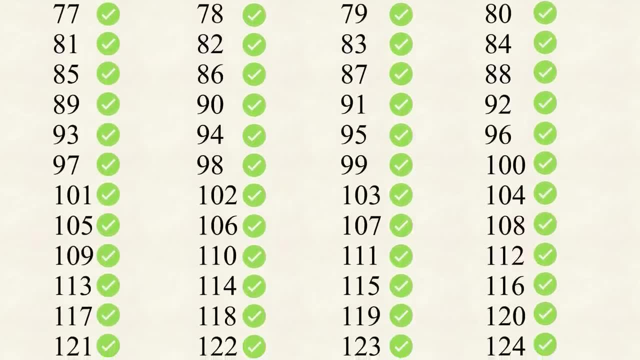 we cannot be sure, like there could be some number, maybe in the millions or trillions which suddenly feel a square-sum property which, I have to admit, would just be awesome. But frustratingly, we do not have any clear insight WHY such arrangements should always be possible. 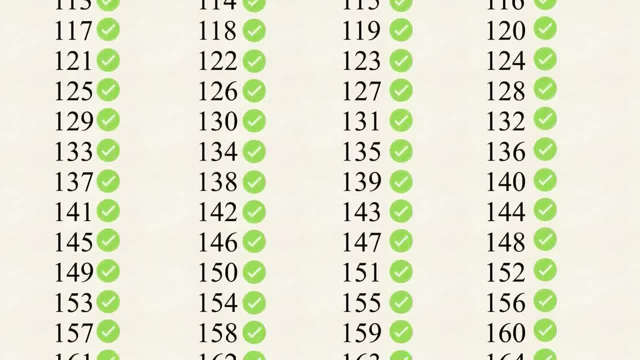 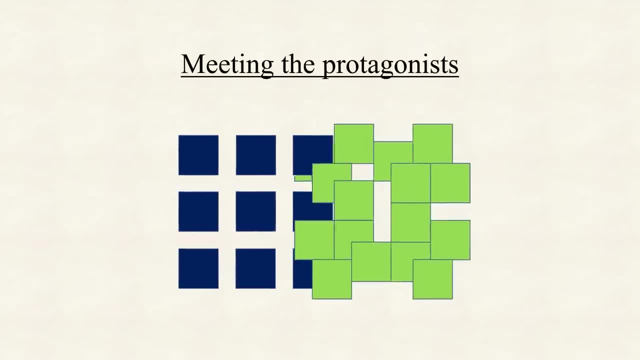 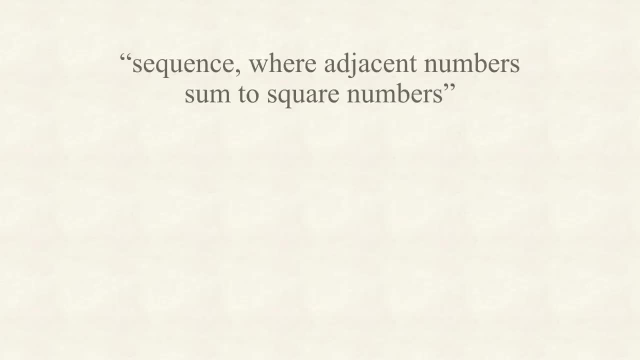 What is needed is a proof, a mathematical reason why such sequences always exist with no exception, and maybe even a way to construct them. So where to start? Maybe we should think in the next video, practical, and admit that the phrase sequence such that the sum of any two consecutive numbers 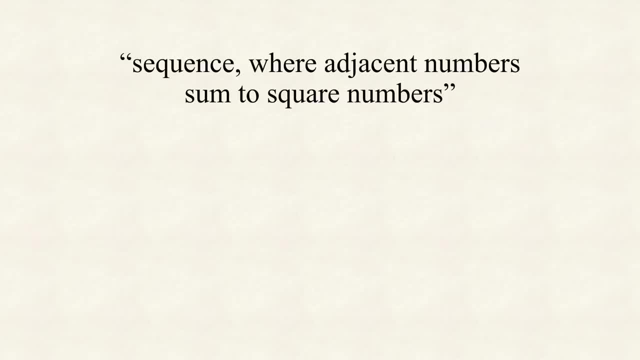 is a square is simply too long. We don't have time for this, So let's just call such sequences regular. For instance, 4, 21,, 15, 1 is a regular sequence, so is 3, 13,, 3, 6 or 5, 11, minus 2.. 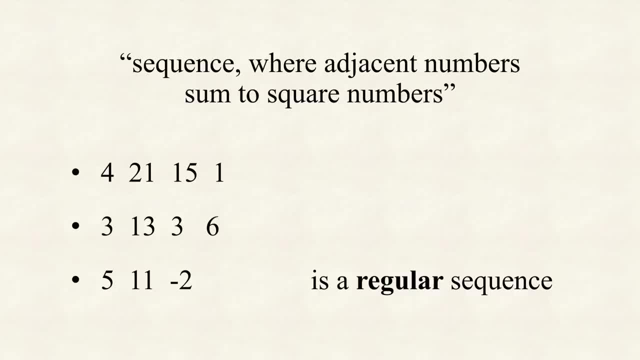 So for now we ignore that eventually we will only have to deal with positive numbers and also want them to appear once in a sequence. Now comes the first critical idea. As we saw in the beginning, finding regular sequences just by searching is tedious. What we would rather have: 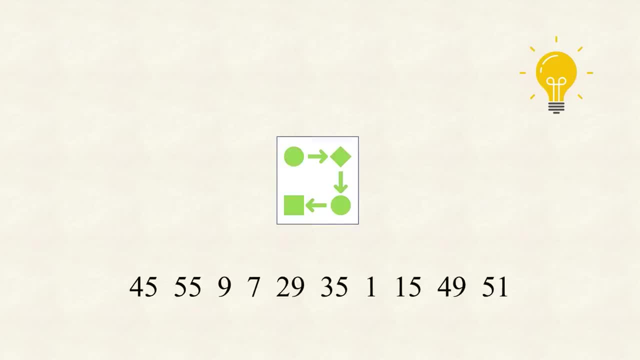 is some way of using regular sequences that we already found to construct new or longer regular sequences. In other words, research for ways to manipulate or transform a regular sequence that gives us a different one. Say: I hand you any regular sequence. There are some ways we can. 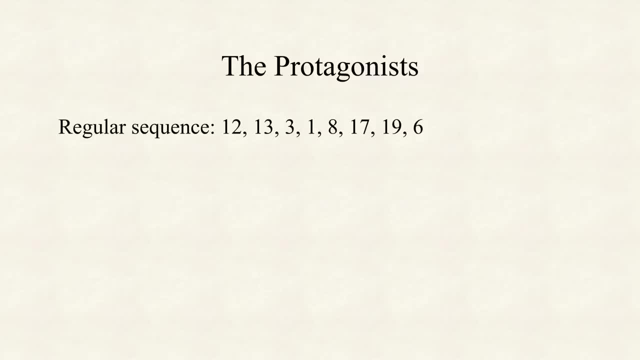 construct regular sequences. For example, we can construct a regular sequence that gives us a new regular sequence without having to do any trial and error. You now have exactly five seconds to pause if you want to find them for yourself. Otherwise, I will start with the first one First. 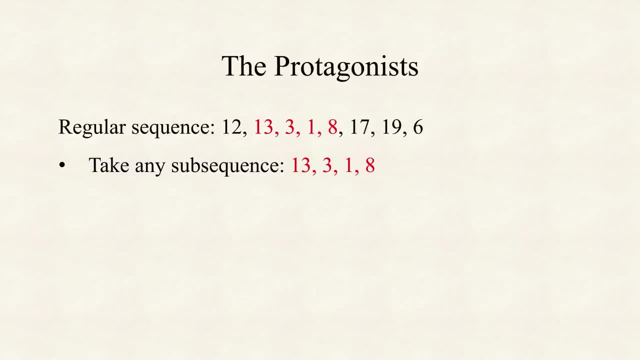 you could simply take any consecutive sum sequence, which is obviously regular again, as we haven't changed the consecutive sums. Not very clever and also boring, so this one will actually not be useful for us. Secondly, you could reverse the sequence. Unfortunately still boring, but this will actually. 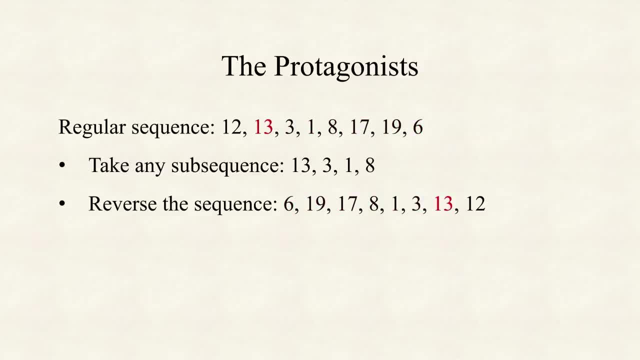 play a role for us Which brings us to the next two transformations. They are what our entire approach will rely on, as they don't just shuffle the existing numbers around. Without the following two ideas, we are doomed and our attempt does not stand a chance. So the third insight is that if 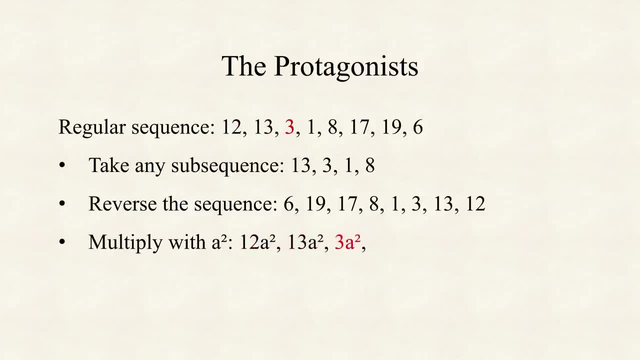 you multiply the whole sequence with any square number a squared, the resulting sequence is still regular. Why is this the case? Take, for example, the first sum, that is, 12 a squared plus 13 a squared. As we started with a regular sequence, we know that 12 plus 13 is a square number In our 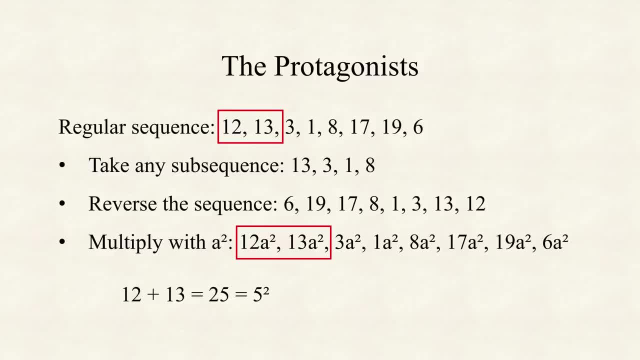 case 25 or 5 squared. Therefore, the new sum, which is 25 a squared, can be written as 5 a squared and is therefore again some number squared. The same argument can be done for the next sum, and so on. And last, what happens when we add some constant to the first number In order to ensure that the 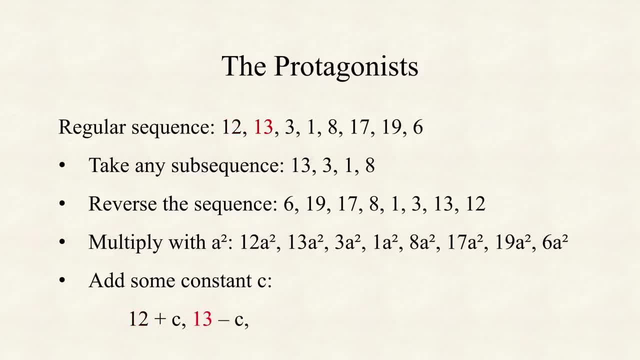 sum of the first two numbers stays a square. we can simply subtract the same constant from the second number, But then we have to add it to the third number to ensure that the sum of the second and third number is unaffected. In total, if we add: 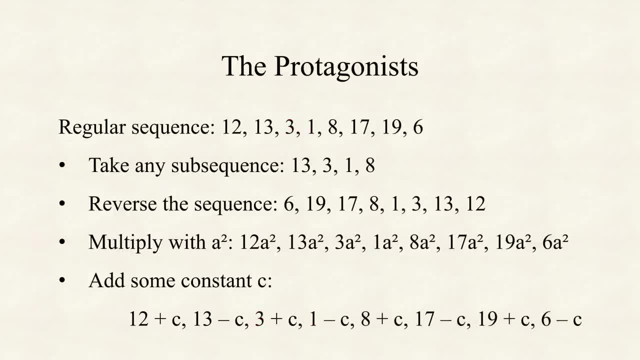 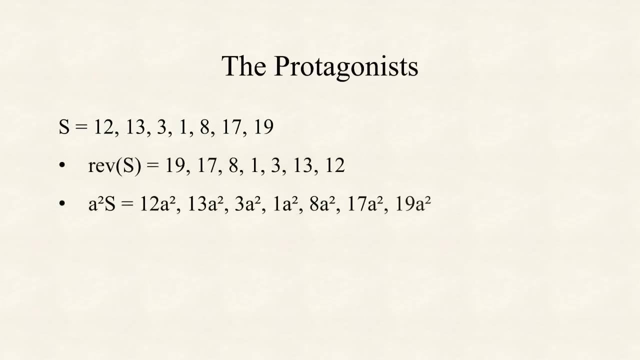 and subtract some constant on and on, the sequence stays regular. In particular, even the sums of the consecutive numbers are unaffected. The last three operators are worthy of getting their own name. If we call a sequence s, then we might write ref s as the reverse of s. Multiplying a sequence by. 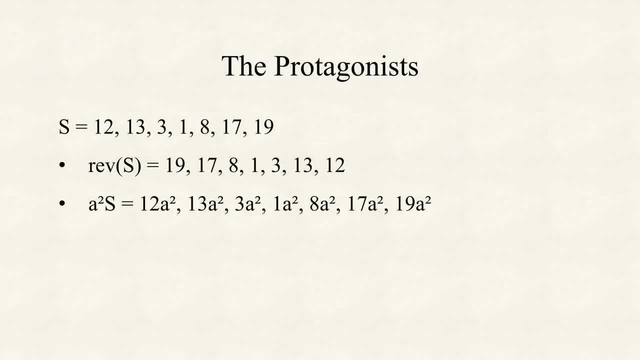 a square number is a square number. If we call a sequence s, then we might write a square number a squared. we can write as a squared s, As the last operator increases or decreases every number. we might call it the shift function and write shift s c, where c denotes the number that is. 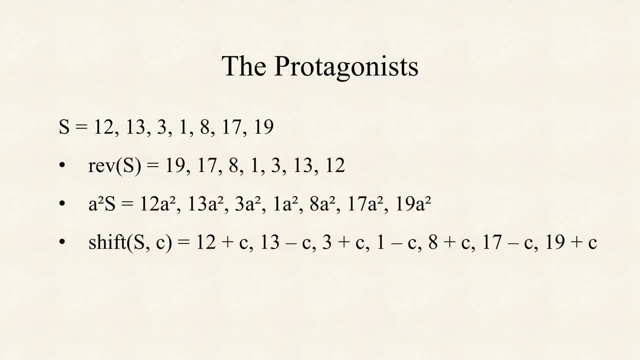 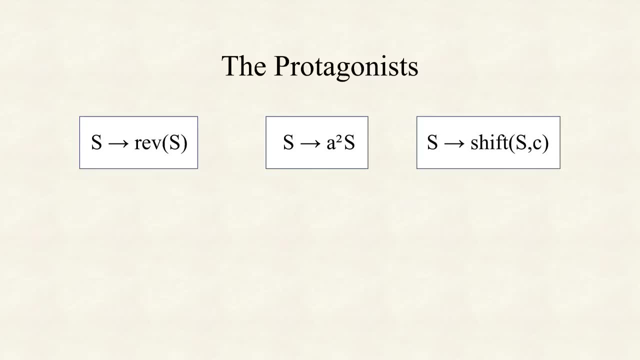 added to the first entry of s and subtracted from the second, and so on, As we now have met our three protagonists. there is one additional fact that I want to highlight. Starting from a regular sequence, we can apply any of the above transformations to get a new one, But since this is again a regular, 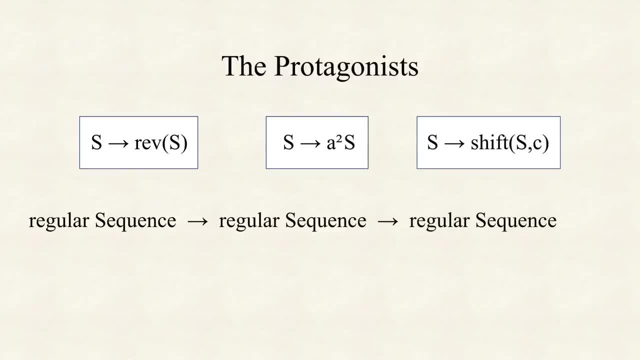 similar. we could then apply a different transformation and then another. The sums of consecutive numbers will always be square numbers, And I think we should point out that, while we are just playing around with the problem, we have made a huge step towards each solution. 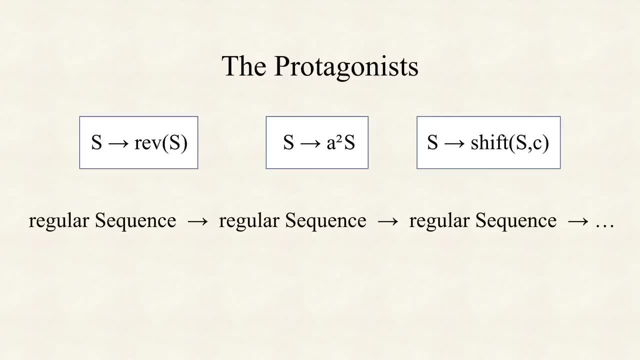 Namely, we found some structure in the thing we want to explore and ways to manipulate it. In principle, we now have all the tools for solving the square sum problem. The rest is like a complicated puzzle where we will try to make further and further progress. 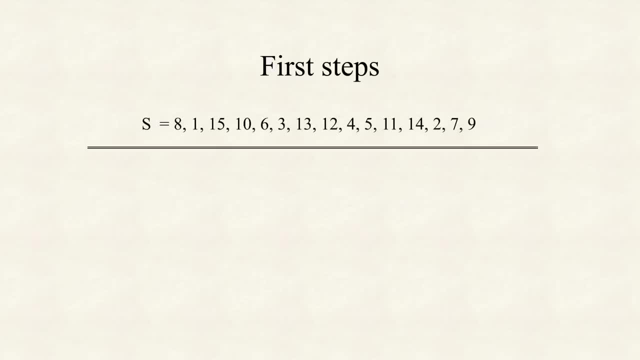 So let's just start with the sequence we had in the beginning and ask the question whether we can apply our transformations to get any closer to solving our problem, That is, create a new solution to the square sum problem. First of all, in order to get larger numbers, we might start by multiplying the sequence. 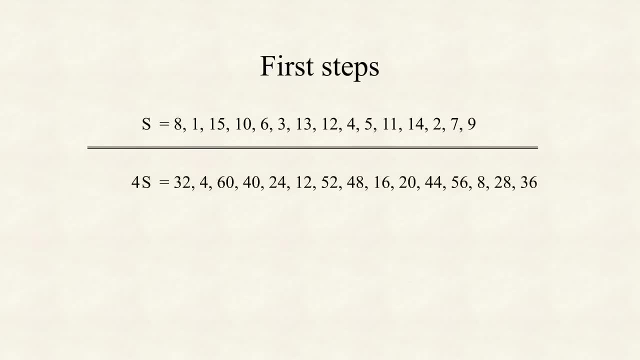 by 4, which is a square number, 2 squared Hence, it gives us a new regular sequence of all multiples of 4 that are less than or equal to 60.. But we already have a tool that can give us more than just a multiple. 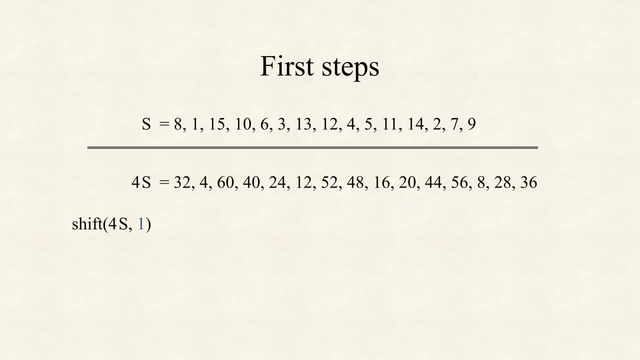 Namely the shift function. If we shift the sequence by 1, that is, add 1, subtract 1,, on and on, we already have a variety of new numbers. Interestingly, we could have also shifted by minus 1,, so starting with subtracting 1.. 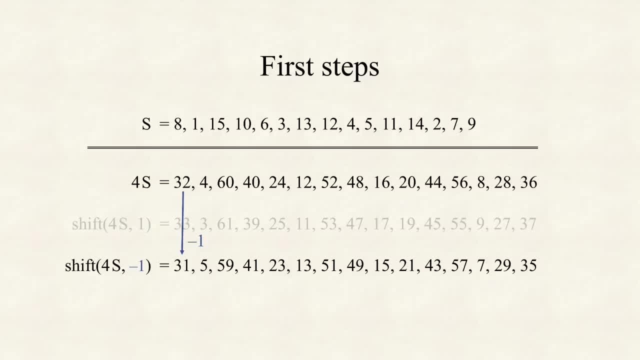 Which again gives us a new regular sequence, And feel free to check that here consecutive sums are indeed always square numbers. Even though we know it should work, I still get enjoyment from actually checking, So we can already package many numbers that are similar. 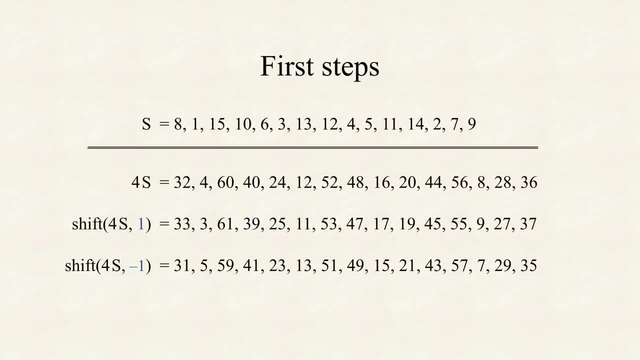 And now we can start to solve the problem. Let's take a look at how to solve this problem. First of all, let's take a look at a number somewhere in between 1 and 60, into three regular sequences, even though they are sort of stand-alone, rather than one continuous string. 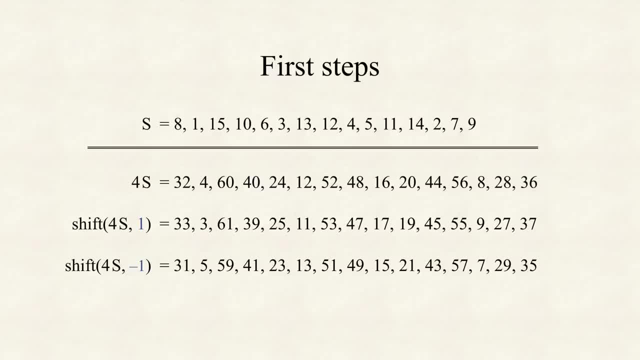 Crucially, we got an extra bonus that none of the new numbers appears more than once, which we know we will need eventually. However, this is the point where we encounter our first obstacle, Namely, as we took care of nearly every odd number up to 60, we only covered half the 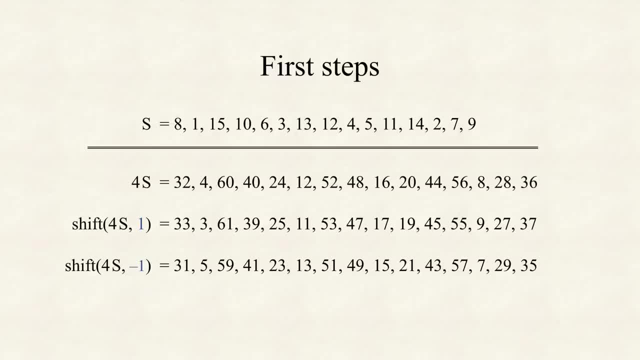 even ones. Sure, we have all multiples of 4,, but other even numbers like 2,, 6, and 10, are not always the same. So let's take a look at how to solve this problem. First of all, let's take a look at how to solve this problem. 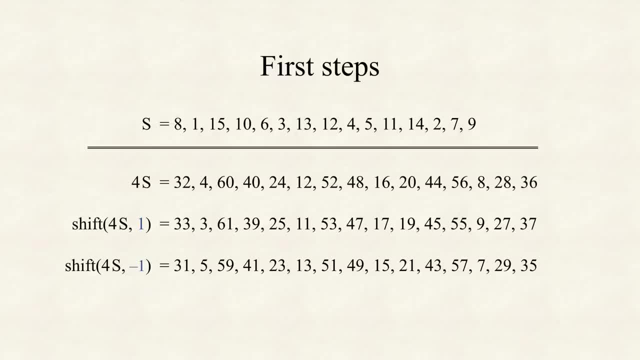 First of all, let's take a look at how to solve this problem. Sure, we got an extra bonus: that none of the new numbers appears more than once, which we know we will need eventually. However, this is the point where we encounter our first obstacle. Namely as we took care of nearly every odd number up to 60,. we only covered half the even ones. Sure, we have all multiples of 4, but other even numbers like 2,, 6, and 10, are not. 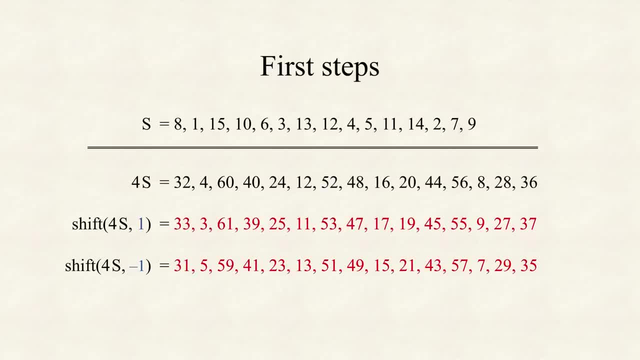 always the same. Sure enough, one could simply shift the numbers by 2, right. Well, yeah, this will give us some of the numbers we are missing, but unfortunately, this time some of them appear more than once. For instance, we can simply shift the numbers by 2, right. 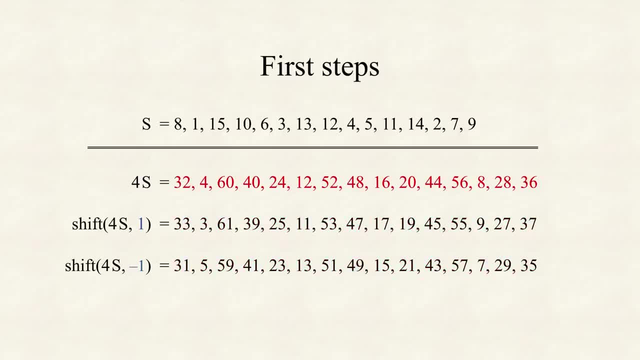 Well, yeah, this will give us some of the numbers we are missing, but unfortunately, this time some of them appear more than once. For instance, we can simply shift the numbers by 2, right, Well, yeah, this will give us some of the numbers we are missing, but unfortunately. 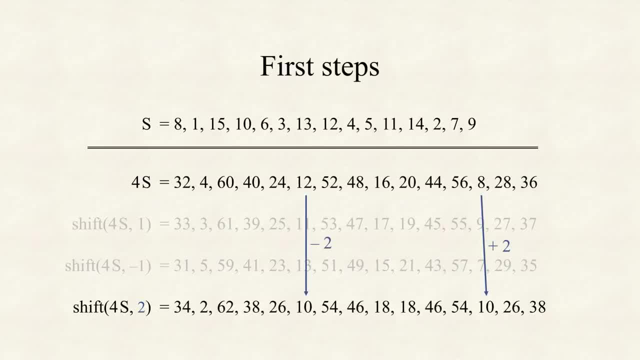 this time some of them appear more than once. For instance, we can simply shift the numbers by 2, right? Well, yeah, this will give us some of the numbers we are missing, but unfortunately, this time some of them appear more than once. 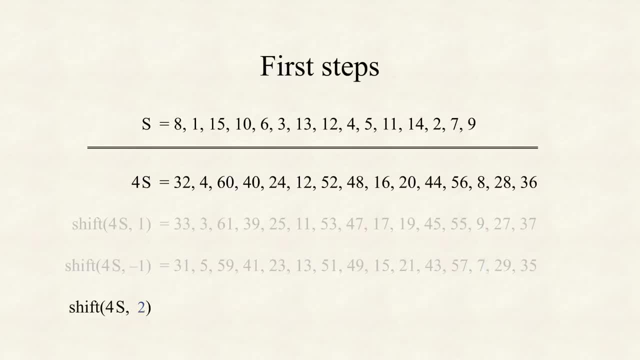 For instance, we got 10 once from shifting 12 minus 2, and again from shifting 8 plus 2.. Is this fixable if we shift by minus 2?? Uh no. Now other numbers appear more than once. Well, 10 does not show up anymore. 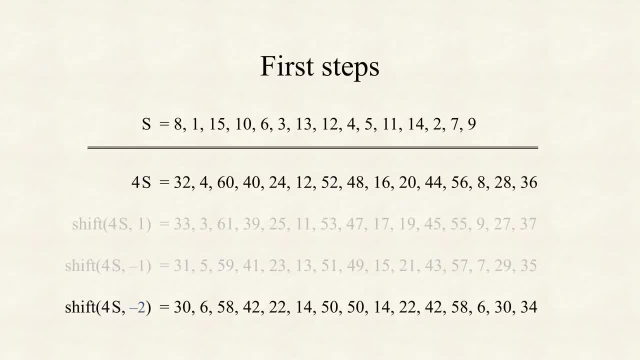 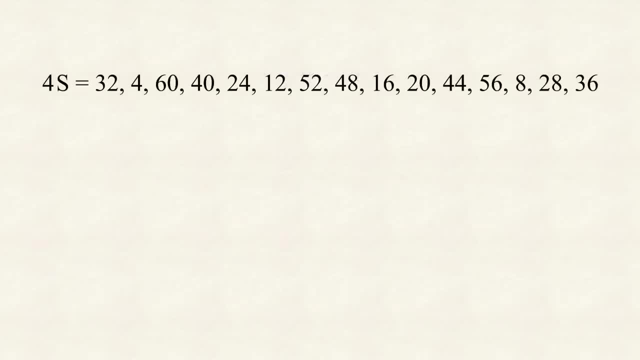 What's going on? Why do these two shifted sequences behave nicely, but the last one won't, and is there a way we can fix it somehow? Well, the reason why shifting by plus or minus one doesn't yield any duplicate, while plus. 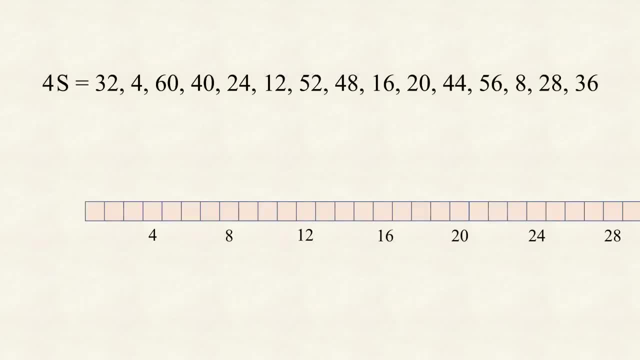 or minus two does, is explained visually. Let's take our sequence that was multiplied before and draw its numbers on the number line. What I'm going to do now is add the shifted sequence with plus one in blue. So some numbers get shifted up by one, while others get shifted down. 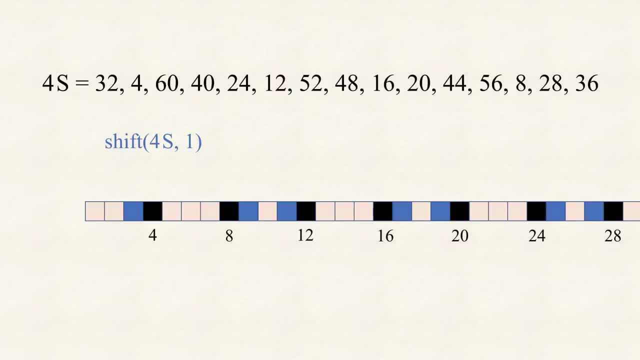 It is quite clear that so far we can't have any numbers more than once. Now let's add shift s minus one. All the numbers that were shifted up by one get now shifted down And note that there is just no way the two points end up on the same number. 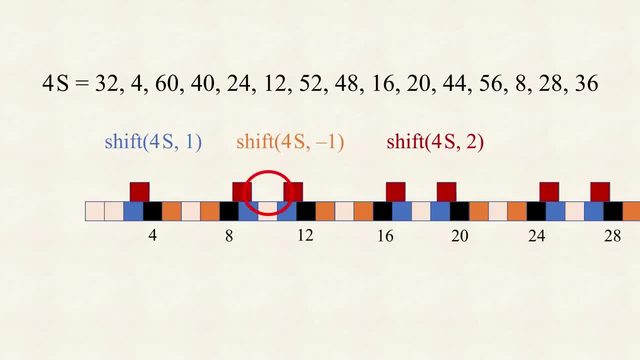 So what's the problem with shift s two? Let's watch. When numbers get shifted by, two intersections can occur. This boils down to the fact that, while every number can only be a distance one away from a single multiple of four, it can be apart from two multiples of four. 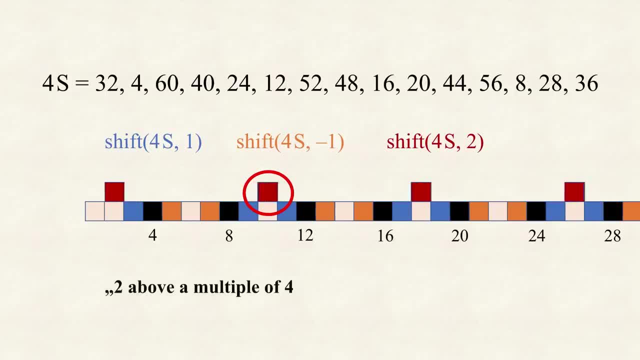 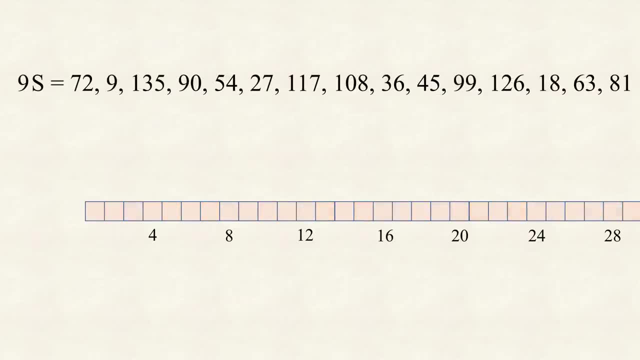 Put differently, the problem is that two above a multiple of four is two below a multiple of four. However, this problem does not occur when, instead of multiplying by four, we multiply with an odd square number, like nine. that is, three squared Again, nine s is a regular sequence. 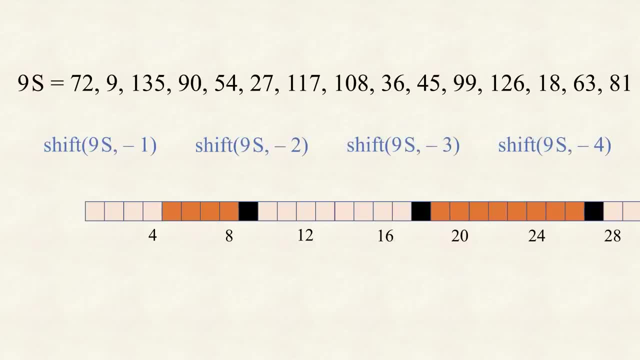 But now, if we consider the sequence shifted by first one to four and then minus one to minus four, we get no overlap whatsoever. Hence every number appears not more than one. Note that here we don't use the numbers from one to four. 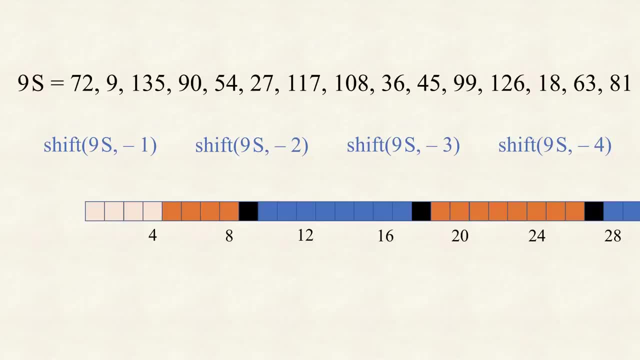 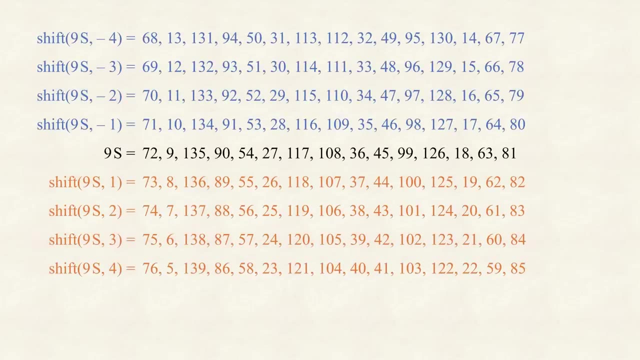 Similarly, the problem with duplicate numbers does not happen when multiplying by any odd square number, like five squared, which is twenty-five, Because there is no number in the exact middle of two consecutive multiples of twenty-five. So we are doing great. By multiplying the sequence by nine and then shifting it from minus four to four, we have 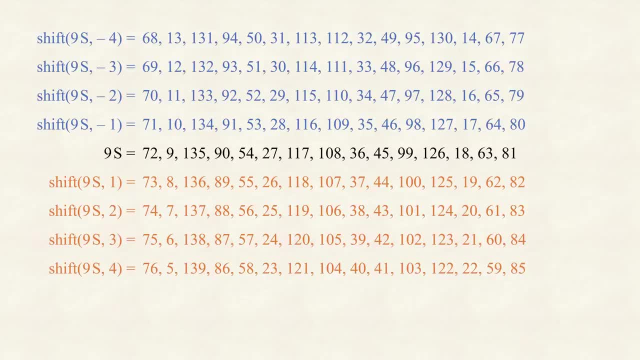 a bunch of new numbers packed in nine regular sequences where no number appears more than once. We would like to somehow link them together to get one continuous string. Also, we would need to include the numbers from one to four somewhere, as they are right. 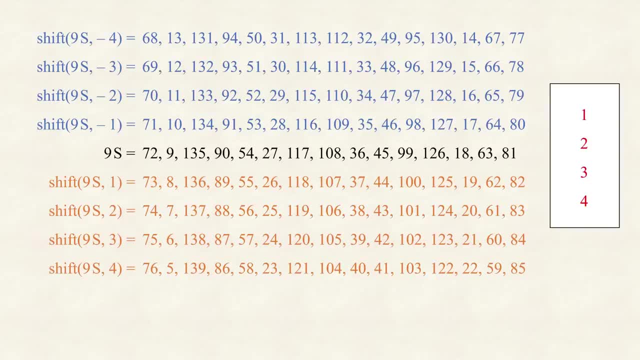 now missing. If we could do that, we would truly have a way to get from one solution to the square sum problem to another. So let's try and start, for instance, with the four. Then we could see that this last sequence ends with seventy-seven, so we might reverse. 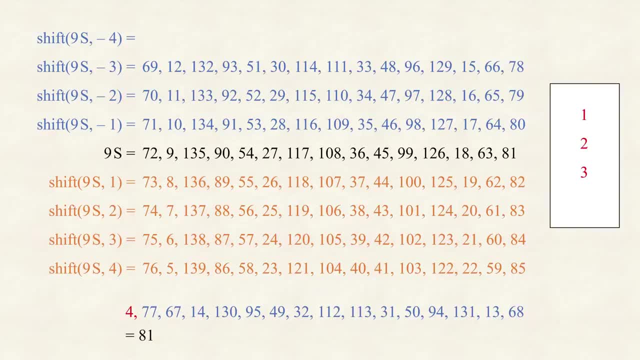 and append it as: four plus seventy-seven is eighty-one a square number. Next may be the first sequence: A sixty-eight plus seventy-six is one hundred forty-four a square number. But unfortunately, this is where our luck runs out. 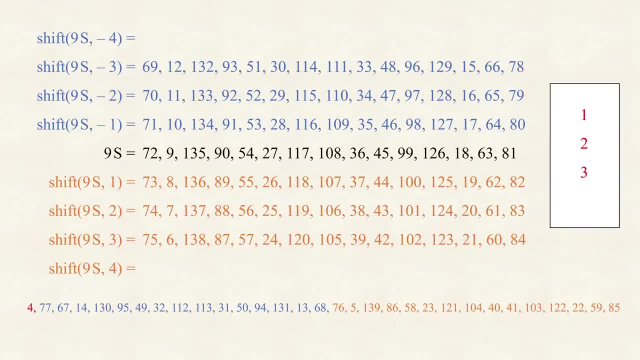 Even if we try longer, we can't do any better. So let's think like a true problem solver and figure out what the problem is and what we would need to do to fix it. Well, something that doesn't bother us is the order in which the numbers in between 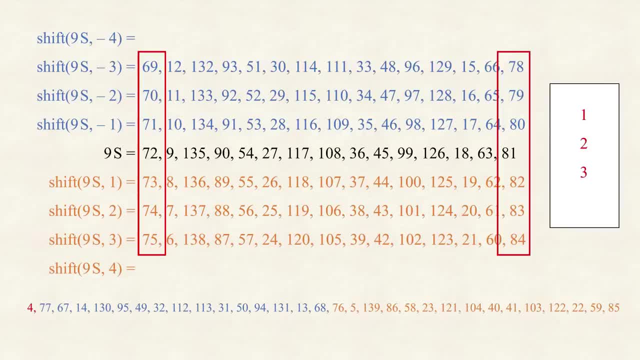 the sequences appear. For us, the only thing that matters are its endpoints, to link them together. And to link these. Well, If we had more numbers, then just one to four- we would have far more options. But the reason we had only four numbers was that we multiplied with nine and shifted. 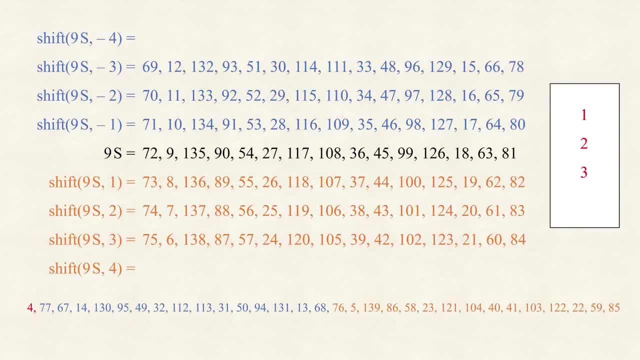 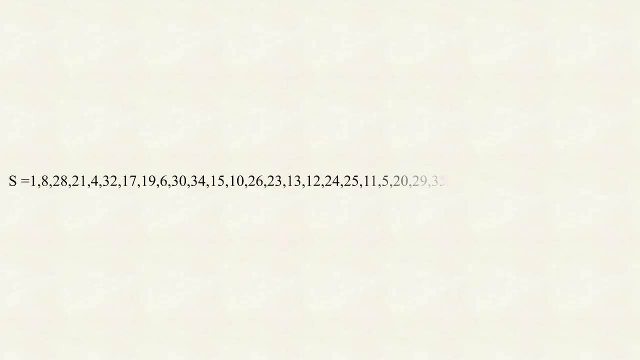 the numbers up to plus and minus four. But we know we could just as easily have multiplied the sequence with twenty-five. That way we get more numbers for linking the sequences together. So let's start this time with this specific sequence. It uses all numbers from one to thirty-five and has one and three. 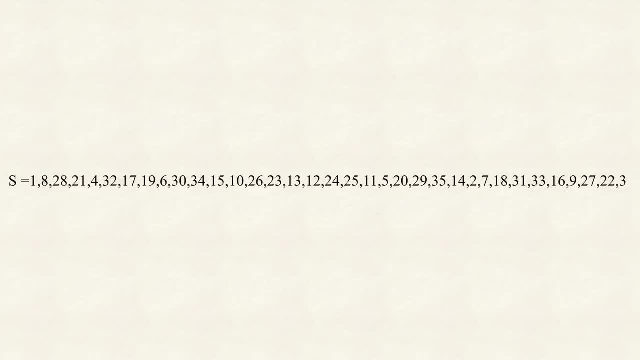 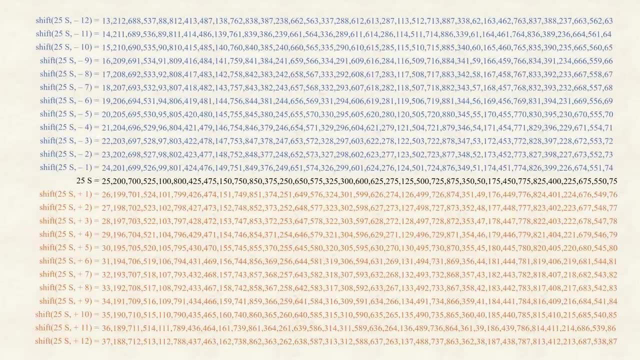 Which might be easier for linking. So we multiply the sequence with twenty-five and now shift the sequence by one, then by minus one, on and on till minus twelve and plus twelve. This way we capture all numbers, from thirteen, which is twenty-five minus twelve, to eight-hundred. 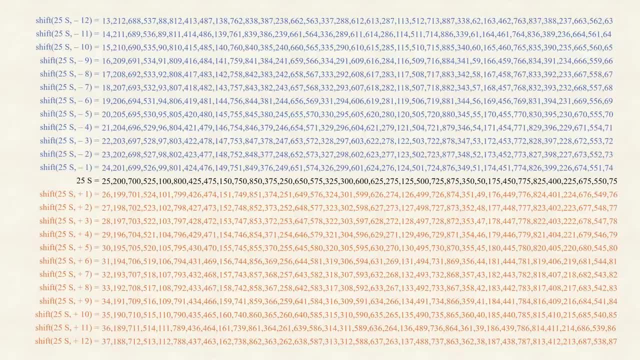 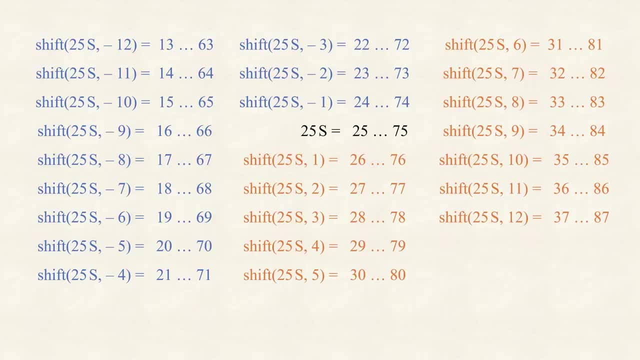 eighty-seven. Not included are the numbers from one to twelve. But before we do anything further, let's abbreviate these twenty-five sequences to keep our sanity and just focus on how they are linked, How they are calculated and what their start and end is. 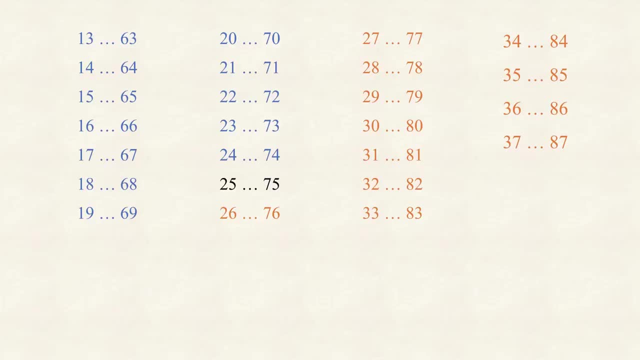 In fact, let's even forget how they were calculated and just focus on their start and end. So we have those twenty-five sequences, as well as the numbers from one to twelve. As it turns out, it is now possible to construct a new sequence. 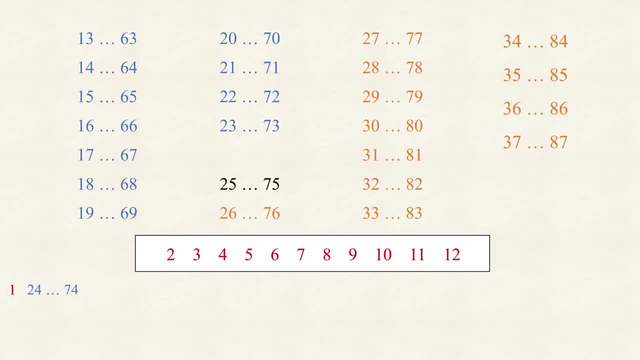 First we could start with one, Then maybe the sequence shifted by minus one, as one plus twenty-four equals twenty-five, a square number. Next this sequence. Now we might add the reverse of this sequence, Then the sequence multiplied by twenty-five, without shifting, then maybe eleven. now 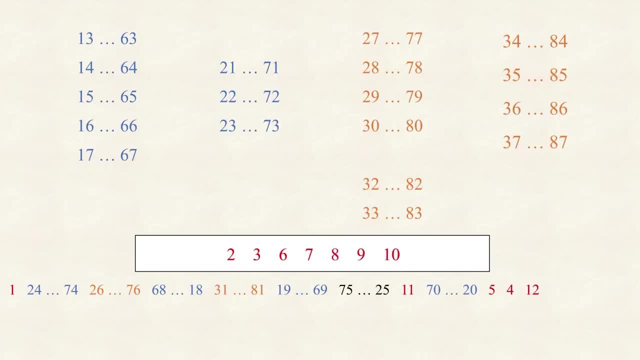 the reverse of that, then five, four and twelve and just all the rest. This way, we can indeed create a sequence involving all numbers, from one to eight-hundred eighty-seven, and we make sure, when joining sequences, that the sums are always squares. 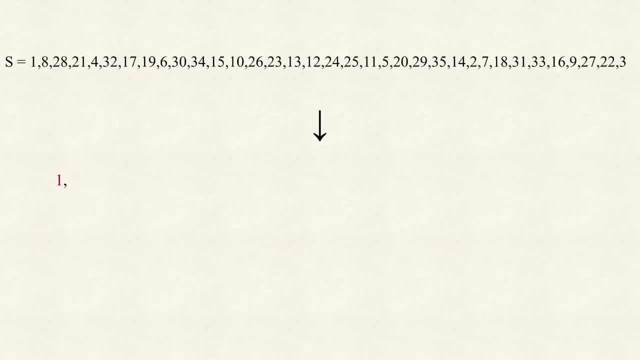 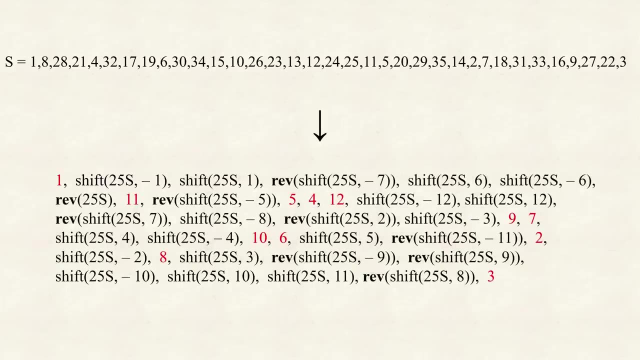 So by taking our initial sequence s, we can get a new sequence by one shift, twenty-five s minus one, And so on, A rule that looks like this. So what does the sequence we just created look like? Well, here it is. 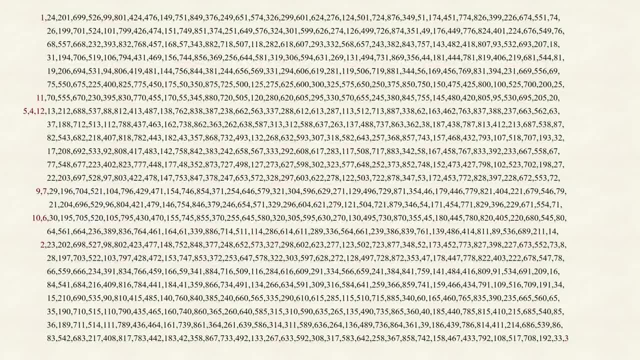 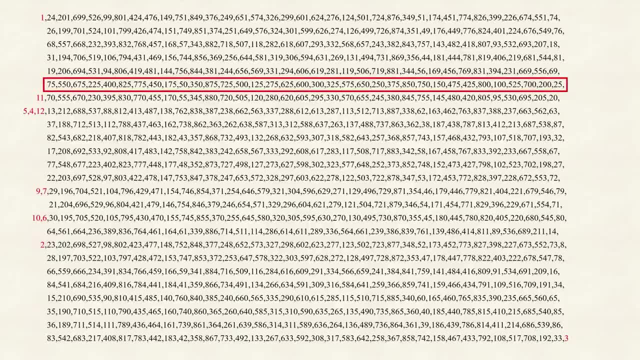 Maybe let's just align it differently to see what happened. First, in red we have the numbers from one to twelve that were used in between the different sequences. Next, the original sequence multiplied with twenty-five is here. here it is shifted by. 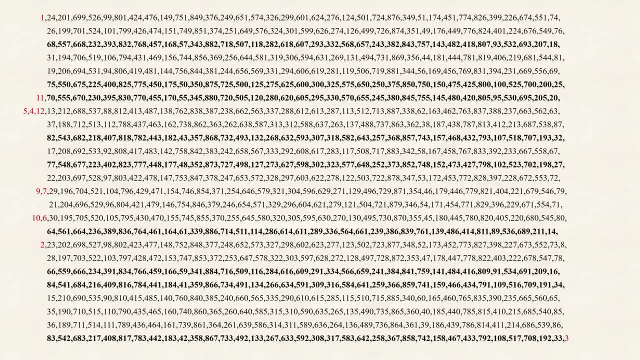 one, and I will also highlight all the sequences that were reversed, If you are bored and don't mind your eyes hurting. just check that this isn't the original sequence. This is indeed a sequence where consecutive numbers sum to squares and no number appears. 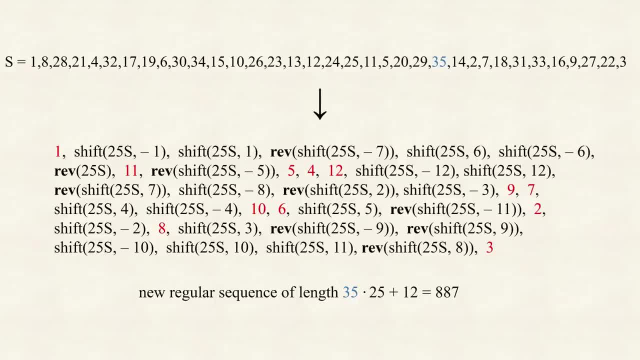 more than once. So this rule, this formula, takes our initial sequence s and creates a new regular sequence. Before s had as largest number thirty-five, so the new sequence has twenty-five times thirty-five plus twelve, which is eight-hundred eighty-seven as the largest number, where 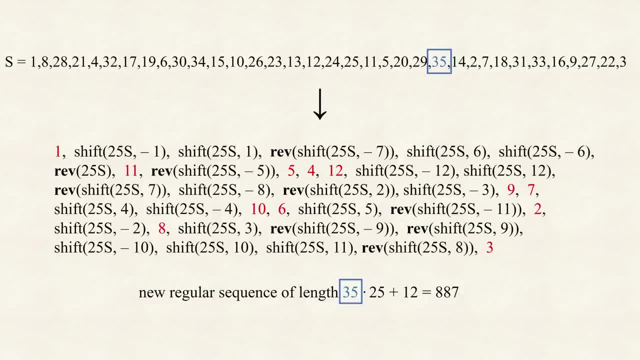 again. the thirty-five is the previous largest number. the twenty-five comes from multiplying by twenty-five and the twelve from shifting up to twenty-five, And so on. So we start with a solution to the squaresum problem, with n equals thirty-five. and now 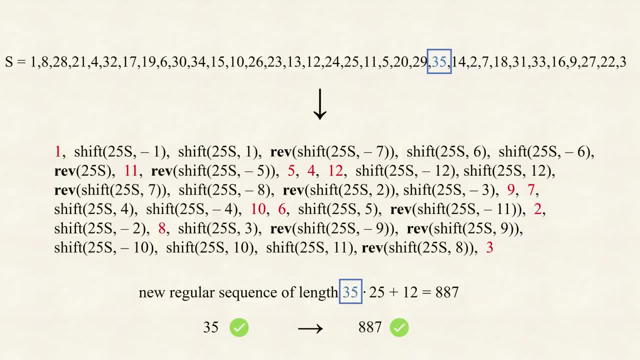 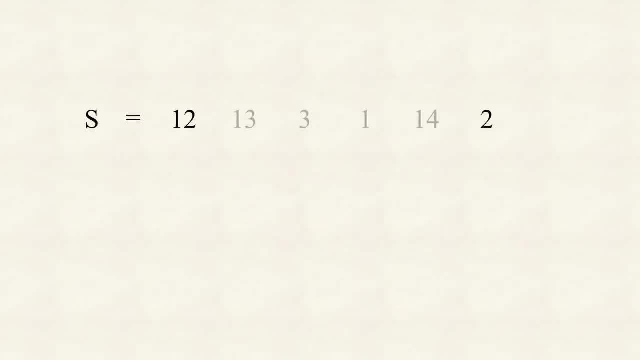 have an additional solution with n equals eight-hundred eighty-seven. However, do you already see what we could do next with this rule? Maybe this helps. Say: we have some sequence and we know its first and last number, Then we obviously also know its first and last number when the sequence gets multiplied. 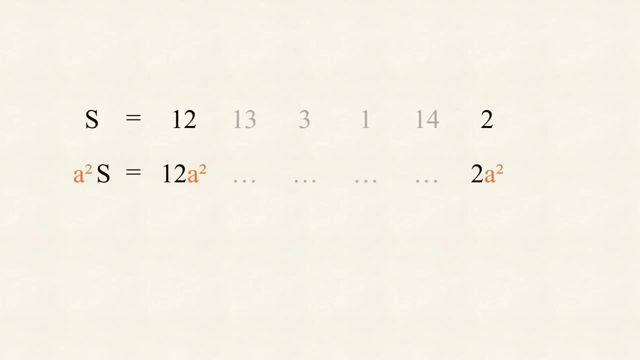 with some square number, As they also just get multiplied. Shifting is more difficult. You see, while the first entry can just be computed by simply adding that c, the last number gets either larger or smaller by c. This depends on whether the length of the sequence is divisible by two or not. 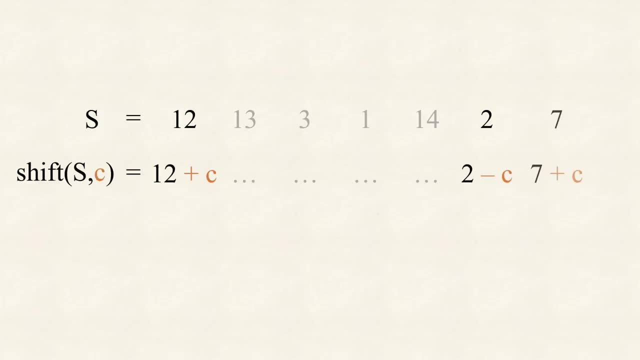 When the length is a multiple of two, we get minus c, otherwise plus c. Well, what I want you to appreciate is that we have full control of the start and end of a sequence, and that those are completely independent of all the numbers in between. 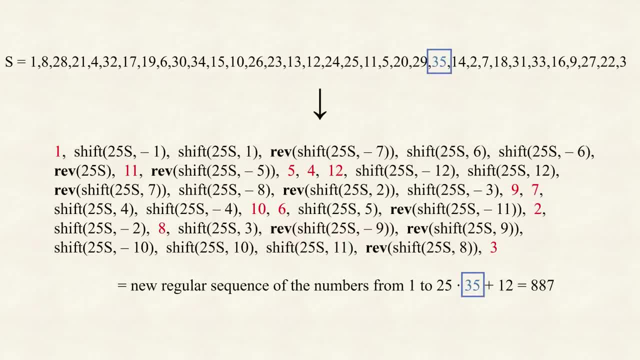 We can see what breakthrough we are about to achieve. This formula can not only be used to extend this specific regular sequence, but rather any regular sequence that starts with one, ends with three and has an odd length to have the same last numbers as our original sequence when shifting. 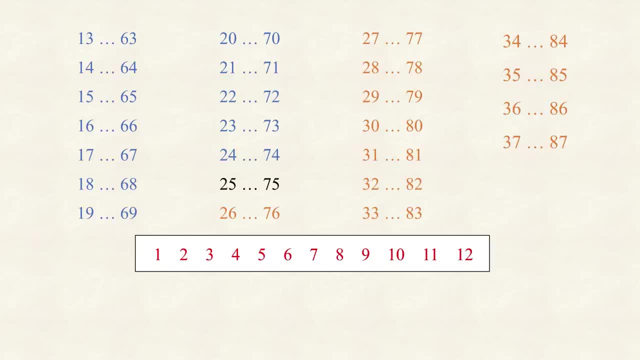 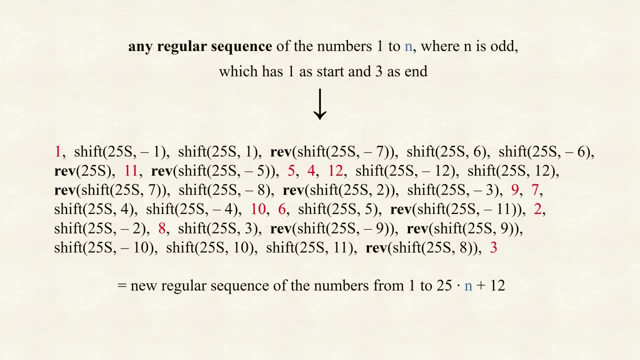 One way to see that this is true is that, while stitching together the shifted sequences, the length of the original sequence, which was thirty-five, didn't play any role As long as the shifted endpoints, after multiplying with twenty-five, are identical. the length 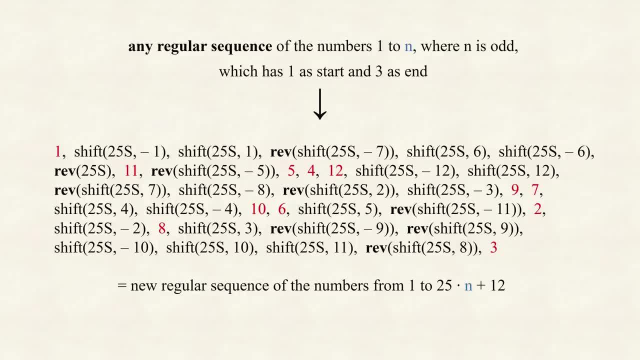 of the original sequence, which was thirty-five, didn't play any role, As long as the shifted endpoints after multiplying with twenty-five are identical. the length of the original sequence, which was thirty-five, didn't play any role, As long as the shifted endpoints after multiplying with twenty-five are identical. the length. 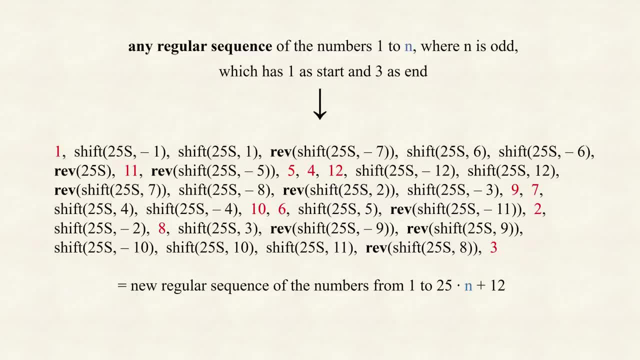 of the original sequence, which was thirty-five, didn't play any role, But this rule not only extends sequences that start with one end with three and have an odd length, but also produces sequences that start with one end with three, and this new 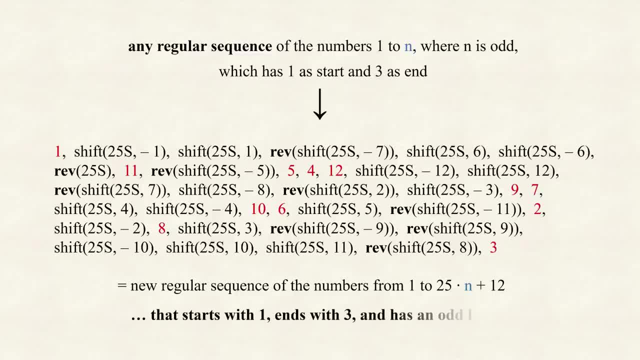 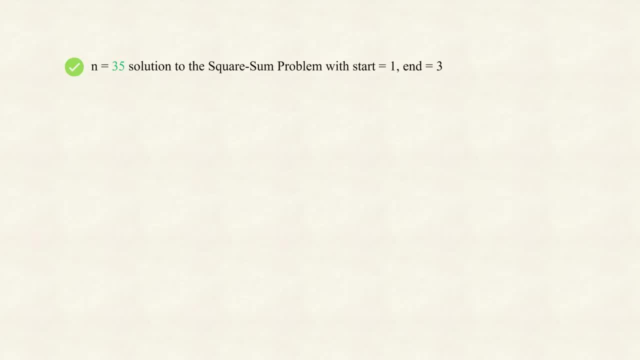 length is indeed always odd, as long as the initial n is odd. So nothing is stopping us from plugging this new sequence back into our formula. Now, what numbers will be contained in the new sequence? Well, the new largest number is always the previous time sequence. 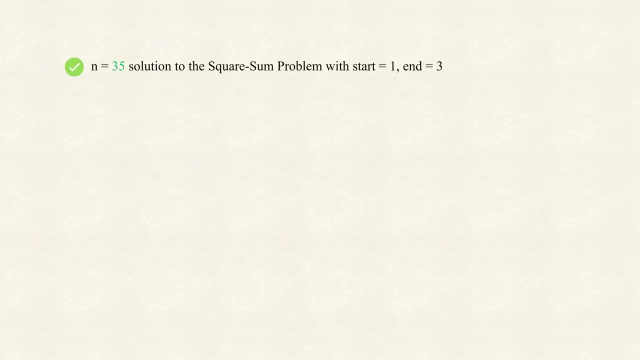 The previous times twenty-five plus twelve. So we started with a regular sequence that had thirty-five as largest number. then the next sequence had eight hundred eighty-seven as the largest number. So if we apply it again, we get a solution to the square-sum problem with n equals twenty-two. 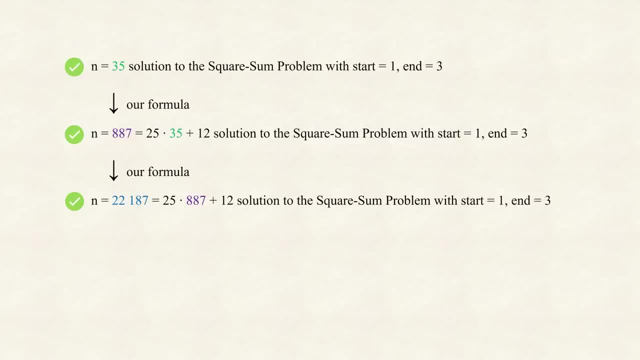 thousand one hundred and eighty-seven. Do it again. We have a solution, for n equals five hundred fifty-four thousand six hundred eighty-seven, And it's hard to stress what a breakthrough this idea is. Suddenly, by finding a simple recipe and a single starting sequence, we get a solution. 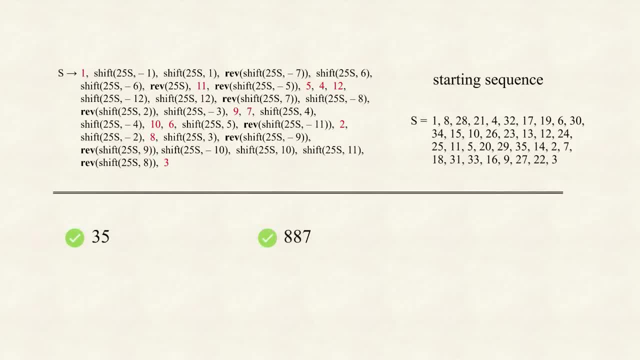 to the square-sum problem for infinitely many numbers, No further work needed. It does not matter how far you wander along the number line. you will at least occasionally stumble upon solutions, and we know why that is and also have a recipe for finding them. 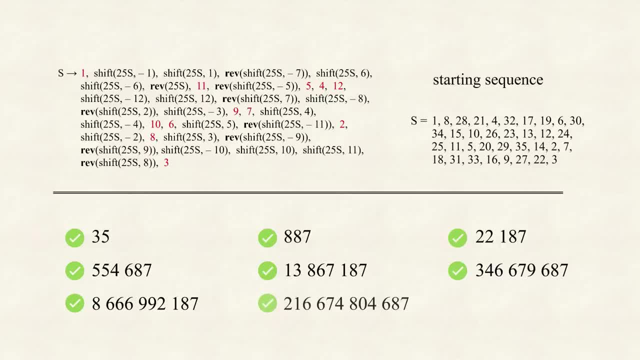 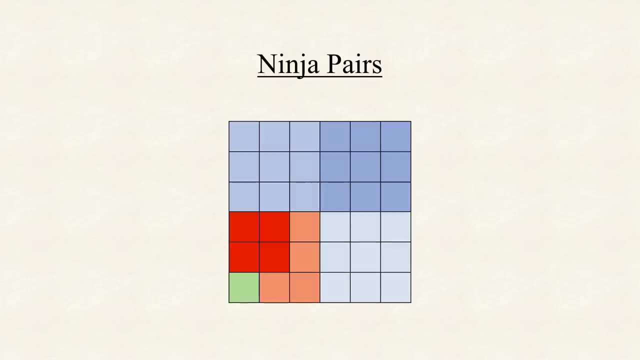 However, it is clear that we are far from done. Even though we can solve infinitely many numbers, there are more than enough that we can't handle. So one last insight is needed to cover all numbers, And unfortunately it is not. It's the hardest one to find. 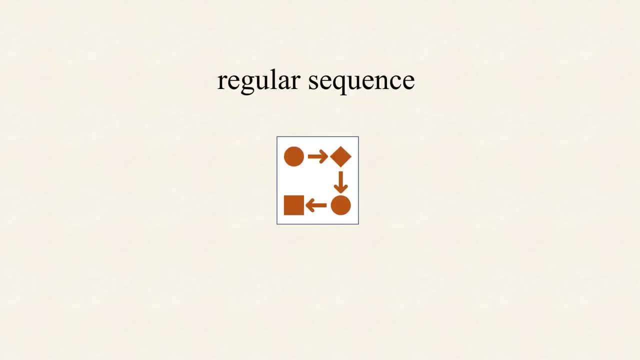 So how far are we from a total solution? Well, we are missing one key idea: Our previous machinery takes only one regular sequence and turns it into another. The key is that when you use a pair of related sequences, you can create new sequences of 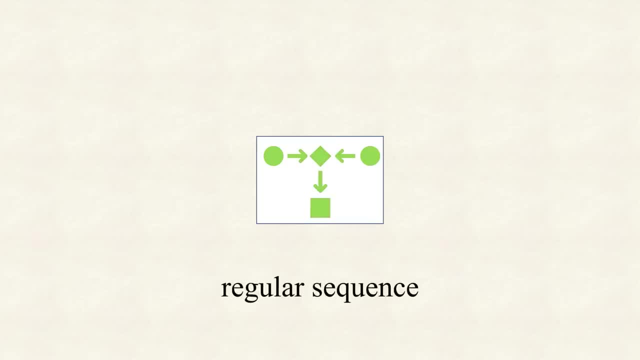 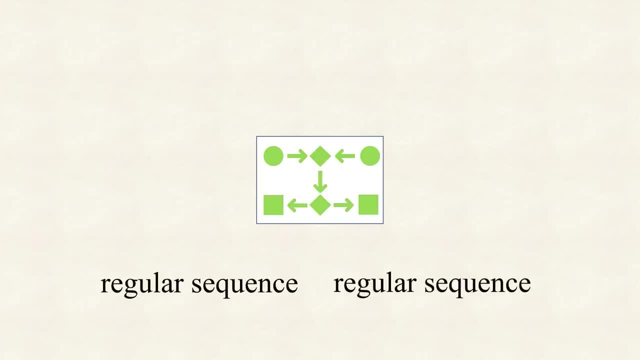 So what we actually want is a way of extending the sequence. So, then, it is more of an acceptation of a long sequence issue, but more of extending pairs of related sequences to different pairs of related sequences. And in order to best introduce these sequences, I'll start with any these related ones. I 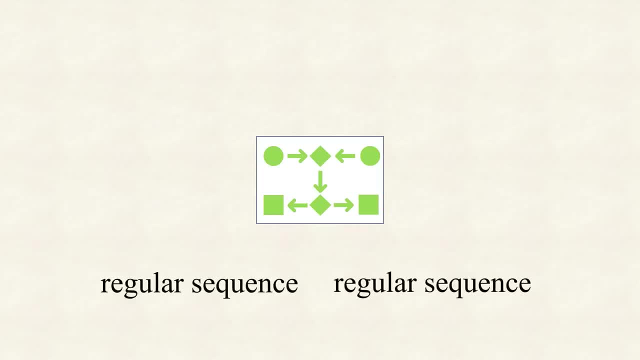 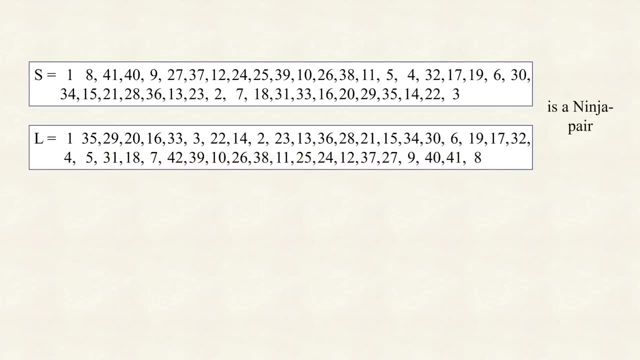 can do, So I'll start with any snack that represents a simple, simple increasing part. For example, the following two sequences form a ninja pair. What makes them special? Four things. First, they are both regular sequences. No surprise so far. 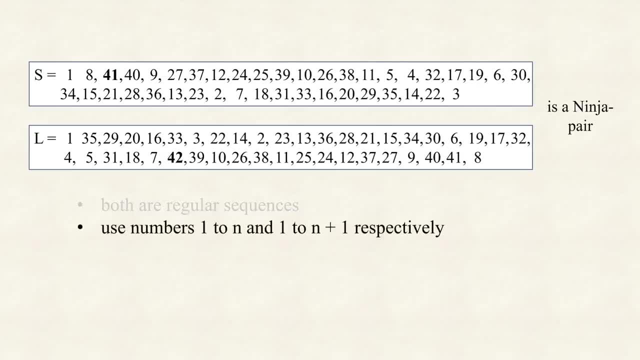 That's one, And another is one that looks like ninja Two, the other a ninja spirit. numbers from 1 to some number, n, while the second contains all numbers from 1 to n plus 1.. In our case, n equals 41, so we will call it a ninja pair of length, 41.. The shorter 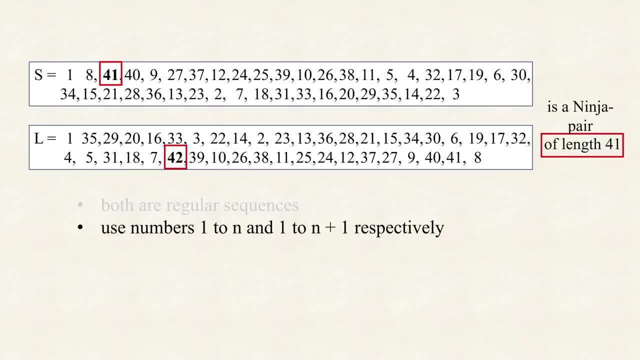 sequence will always be called s for short, the longer l for long. Third, both sequences start with the number 1, and the sequence with an even length has 8 as final number, while the other ends in 3.. This part is also not too surprising, as 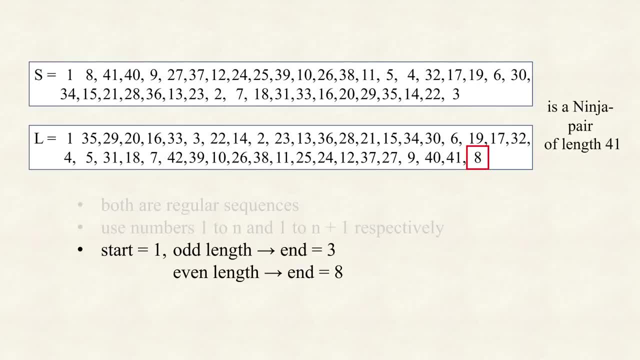 we already understand the importance of first and last numbers. Last, every number that appears in the first sequence in an even position also appears in the second in an even position, and similarly for numbers in odd positions. Look, if we color every other number in both sequences, every number that occurred red in the first. 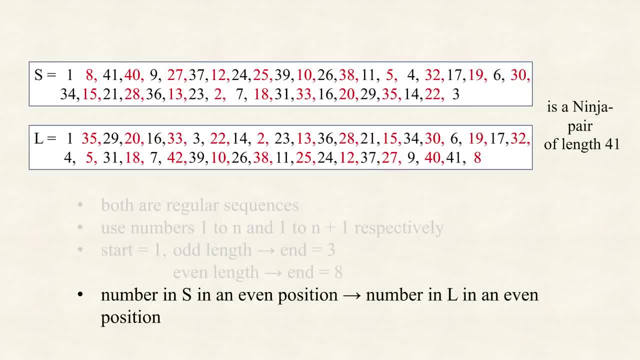 sequence is also red in the second sequence. One might already guess that this has something to do with shifting the sequences. So those are the four criteria for two sequence sequences to form a ninja pair. They are regular and use all numbers from 1 to n, and 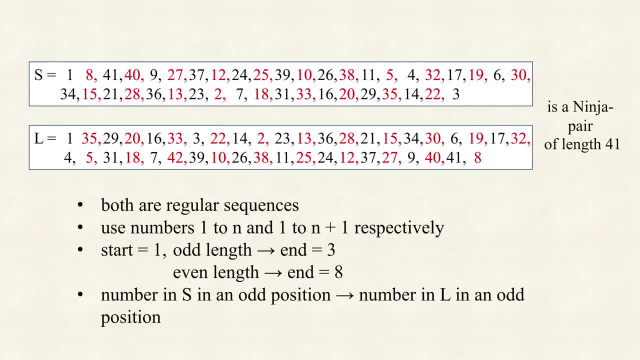 n plus 1 respectively. they start with 1,, end either with 3 or 8, depending if their length is a multiple of 2 or not, and have this property with odd and even positions. And why do we call them ninja pairs? For absolutely no reason other to make them sound exciting. 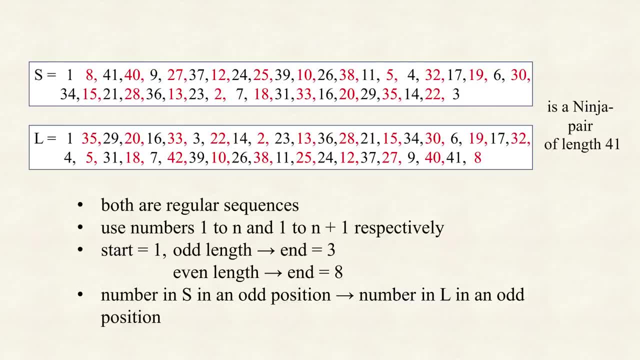 So for now, let's just go with this definition, and especially that final point which we will address later. As it turns out, one is now able to construct a ninja pair, and it is possible to construct one ninja pair from another, much in the same way as before. However, this time we will 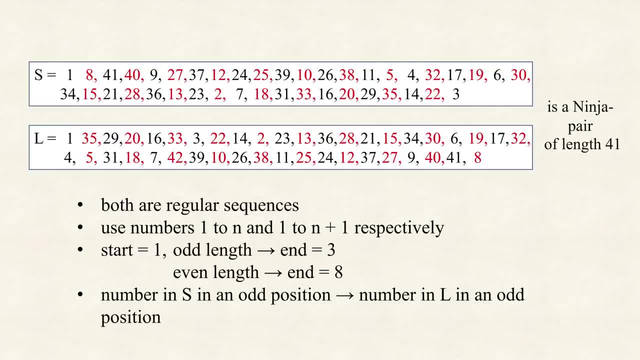 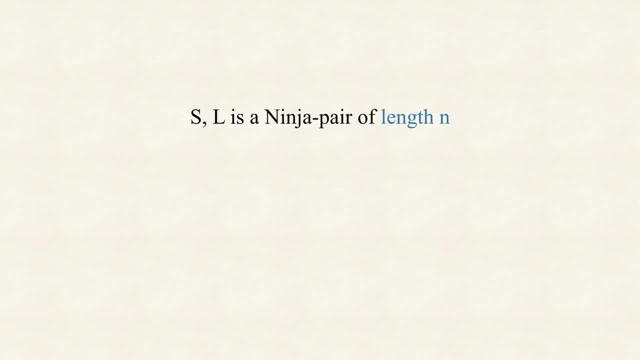 not be multiplying with 25, but instead with 7 squared, so 49,, which is the next biggest odd square number. Say, we have two sequences that form a ninja pair, s and l, where again s is shorter by 1 and consists of the numbers from 1 to n. Then we can use a formula to: 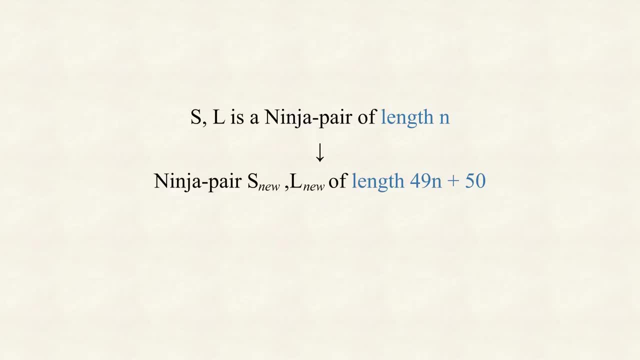 get a ninja pair of length 49n plus 50, and even though there is not really a point in showing you the precise formula, we can use this formula to get a ninja pair of length 49n plus 50, and even though there is not really a point in showing you the precise, 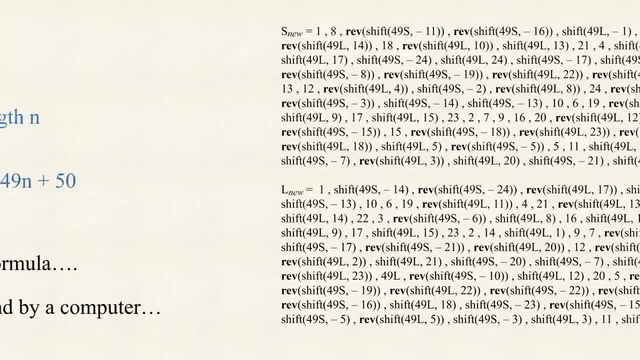 formula. we can use this formula to get a ninja pair of length 49n plus 50,. and even though there is not really a point in showing you the precise formula, as it suffices to know that it exists rather than its exact form, still here it is. 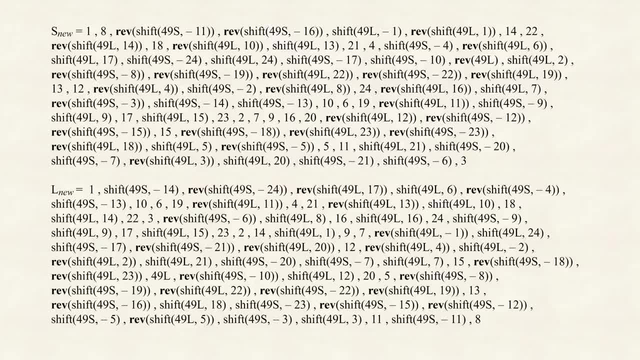 This is the way to construct a Ninja pair: S and l. Actually, this very formula only works when n is odd, but don't worry, one can just as easily find a formula when n is even. so, that's nothing to be concerned about. 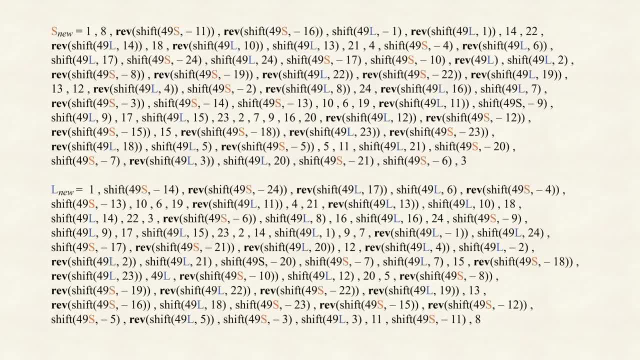 So the bonus is that we can now mix the first and second sequence to open up new possibilities. And here the last point of ninja pairs is important. Take for instance these 2 sequences: Once 49S is shifted down by 11, and then 49L is shifted up by 11.. 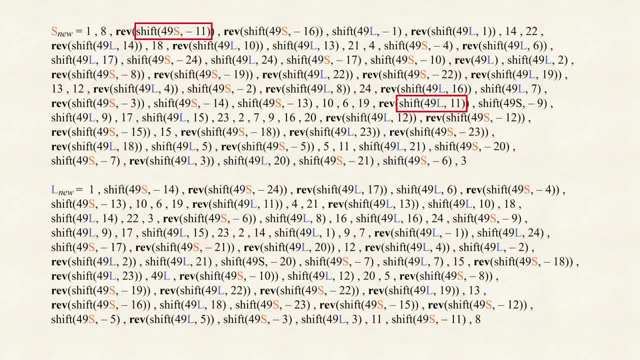 If S and L were any arbitrary pair of sequences, it would be quite likely that there is a number that is contained in both of those shifted sequences, hence breaking our entire process. This is reminiscent of the problems we had earlier, that numbers can appear more than. 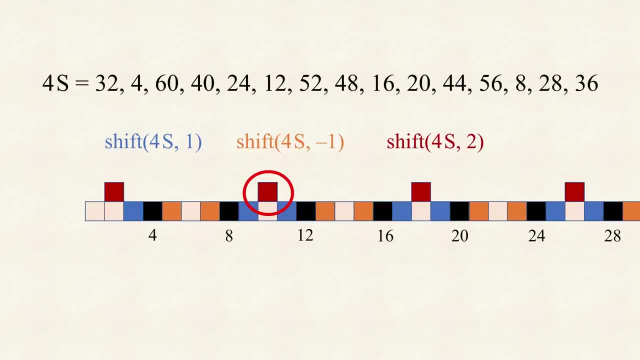 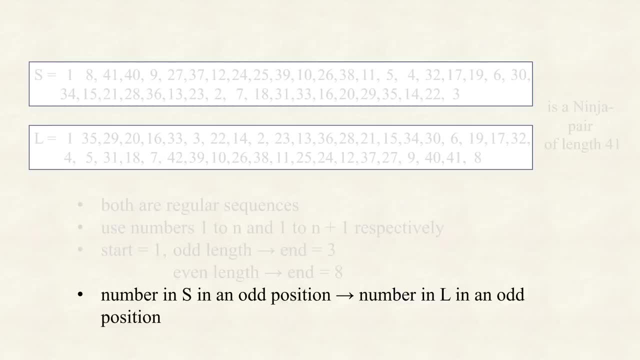 once after shifting. This is why we need our fourth condition on ninjas. It perfectly ensures that such repeated numbers cannot occur. That's the reason we not only want that fourth property, but rather are forced to use it. However, there are more formulas for extending ninja pairs than just this one. 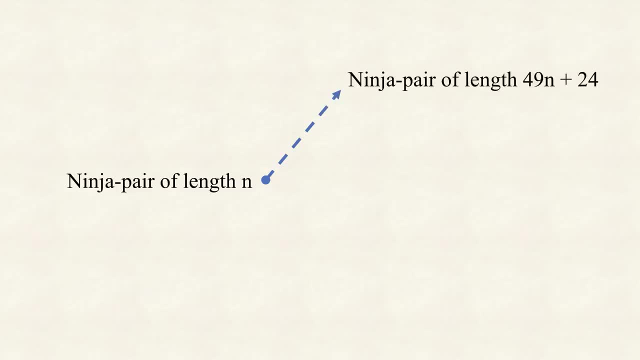 In fact there is one that constructs a ninja pair of length 49N plus 24, when given a pair of length N, Similar for 49N plus 25, 49N plus 26,, on and on till 49N plus 72.. 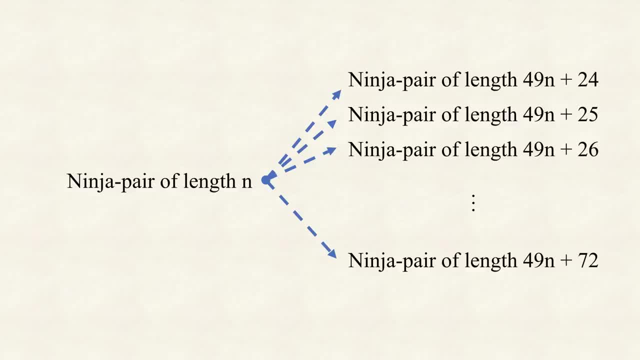 Again, always with a different version for odd and even numbers. In total, this collection consists of 49 different ways of getting new ninja pairs from a single starting pair, which already feels like we are close to actually solving the square-sum problem. Now, even though the definition of ninja sequences is quite constrained, they are still quite 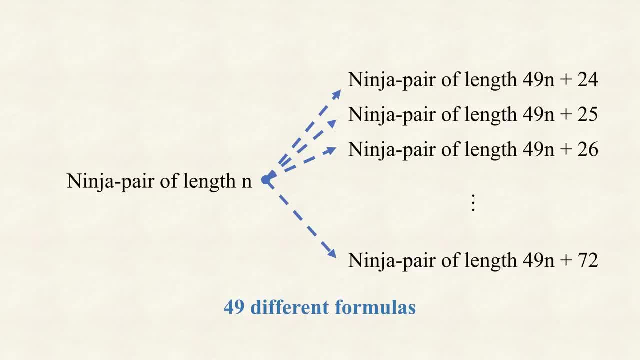 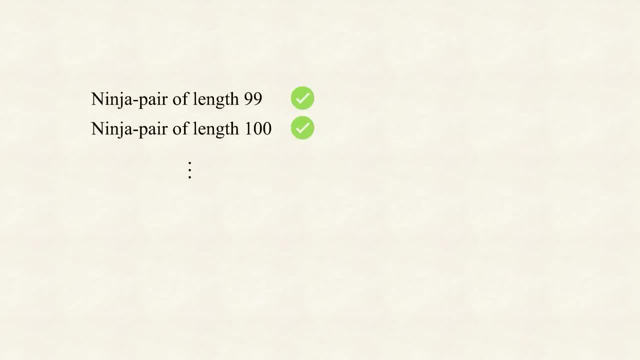 abundant. True, when N is small, they just don't exist. However, we saw that for 41, a pair exists and, more importantly, for N equals 99,, 100, up to 4900, there always exist ninja pairs. 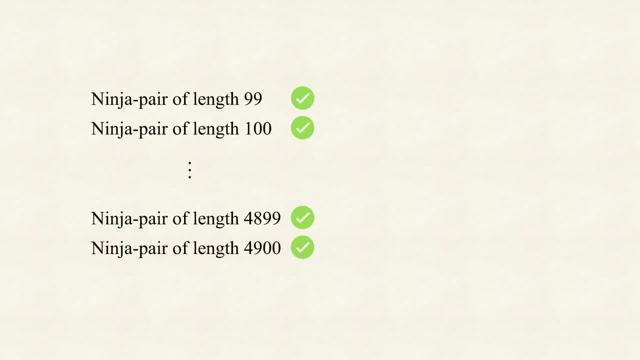 So this is the definition of ninja sequences. But what about 4901?? Well, it can be written as 49 times 99 plus 50. There exists a ninja pair with N equals 99, and we know how to extend it by 49N plus 50,. 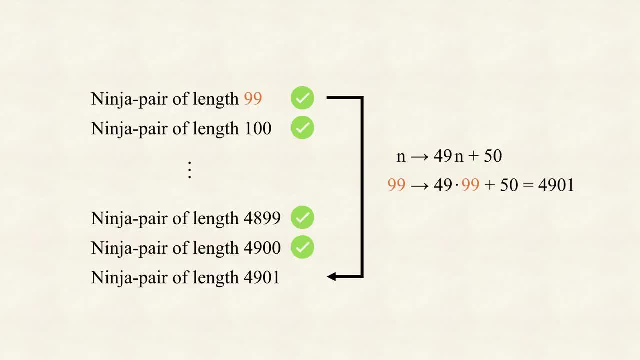 so there has to be a ninja pair with N equals 4901.. Similarly, we know how to extend that sequence by 49N plus 51, so a 4902 ninja pair exists as well. In total, the solution for N equals 99 can be used in the following way: 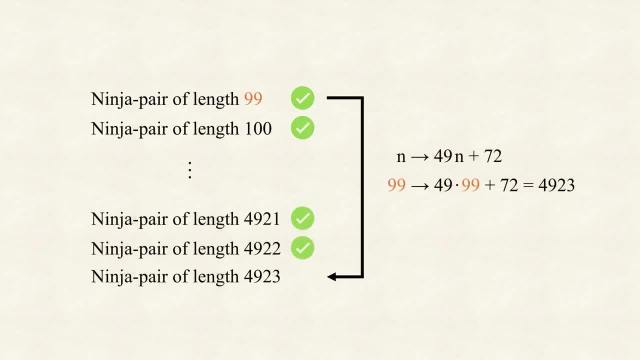 For example, if we want to extend a ninja pair with N equals 99,, we have to extend a ninja pair with N equals 4901.. This is used for creating ninja pairs up to 4923.. However, 4924 is not a problem at all, as we can take the solution with N equals 100. 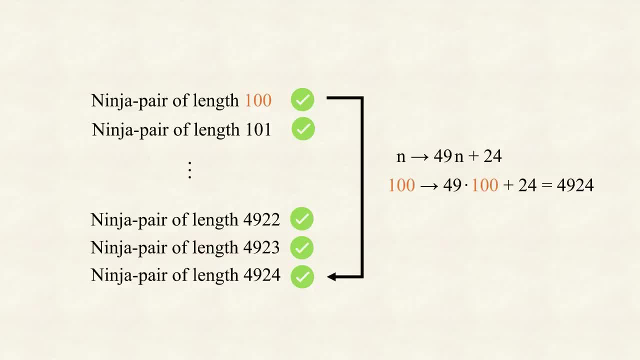 and get 4924.. Each initial solution can be used to create 49 new ninja pairs using our collection of 49 formulas, at which point the next ninja pair can take over to create the following 49 ninja pairs. So this procedure goes on and on, as every new pair can be constructed from an already. 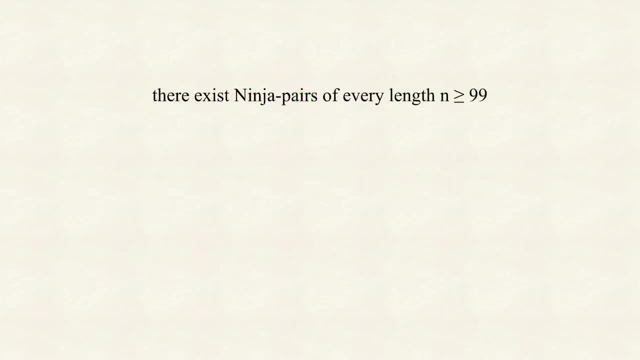 existing ninja pair and the chain cannot break. And just like that, for every N from 99, there exists a ninja pair of length N, And as this pair consists of regular sequences, the square-sum problem is solved for N greater than 99.. 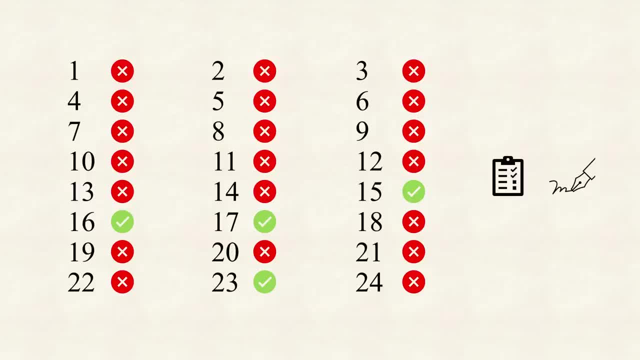 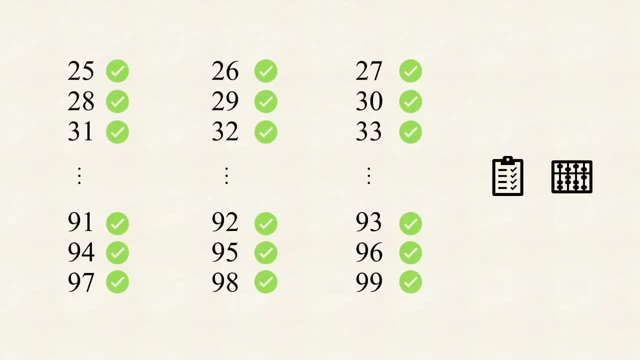 This is how to solve Matt Parker's square-sum problem For small n. sometimes solutions exist, sometimes they don't. Then, from 25 to 99, there is always a solution From 99 to 4900.. The computer even finds a solution. 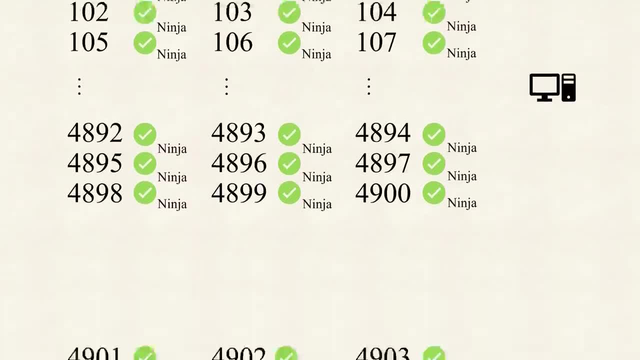 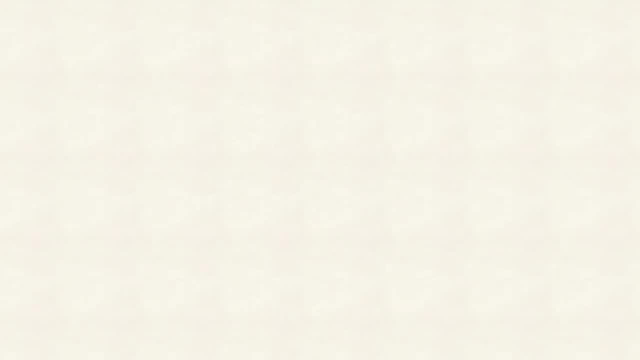 The problem is solved. It finds ninja pairs And from then on, we can, one by one, construct for every additional number a ninja pair to ensure that the sequence of ninja pairs does not end. This very proof was posted online, together with a file including all those initialed. 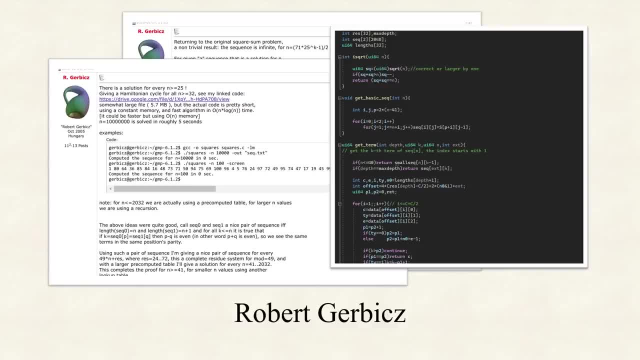 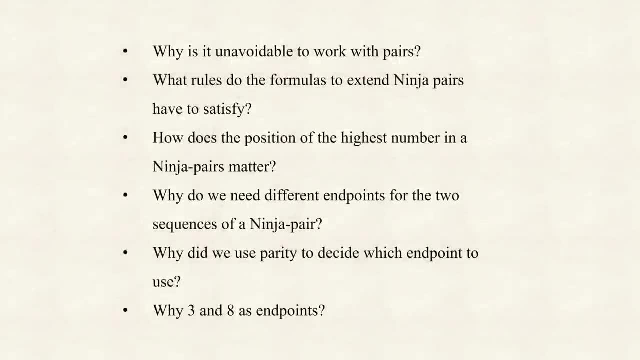 ninja pairs and formulas to extend them, as well as a program that verifies that they indeed are valid solutions. I certainly skipped over some details. however, it is safe to leave them out of a video as they don't offer any additional insights. 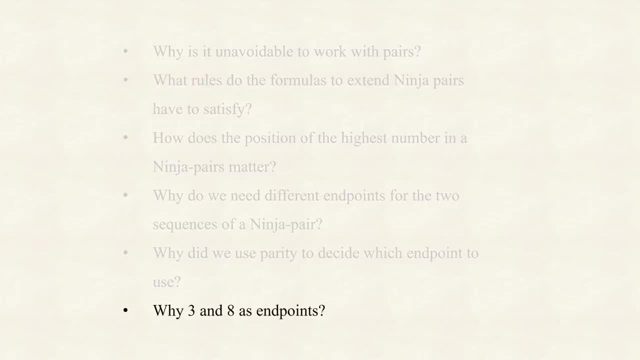 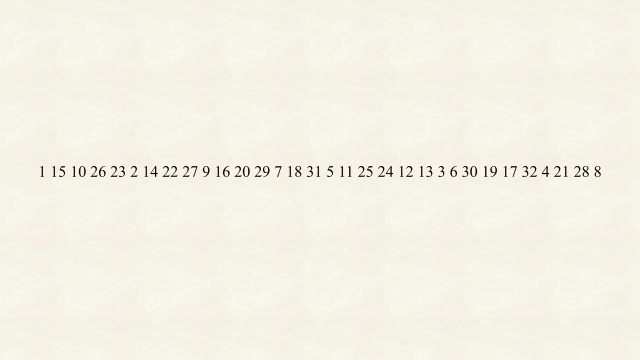 There is only one worthy of being pointed out, which is why we took the numbers 3 and 8 as endpoints. Well, if you have a regular sequence that starts with 1 and either ends with 3 or 8, you can connect its start and end, as they also sum to a square number, resulting in. 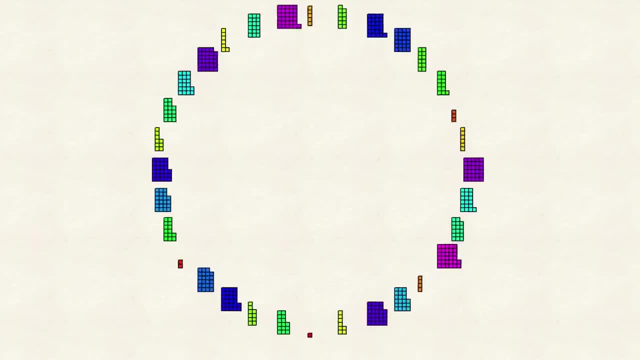 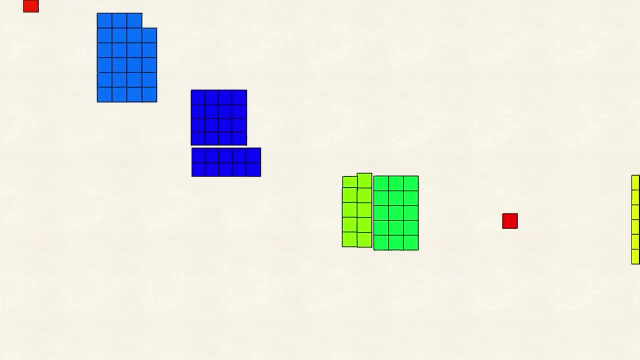 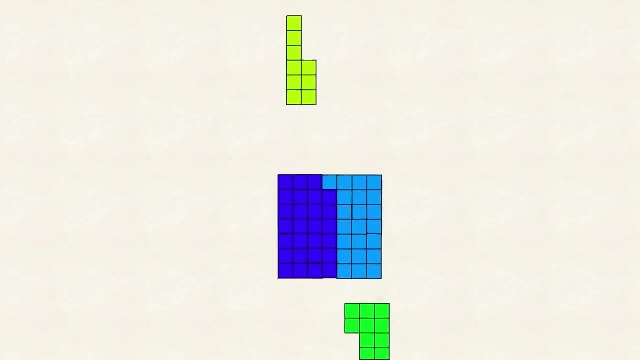 an even prettier animation. Thereby our method not only generates regular sequences, but rather regular cycles, And as it turns out, such regular cycles always exist when N is greater than 31.. So I hope I showed that virtually every step can be motivated by precisely pinning down. 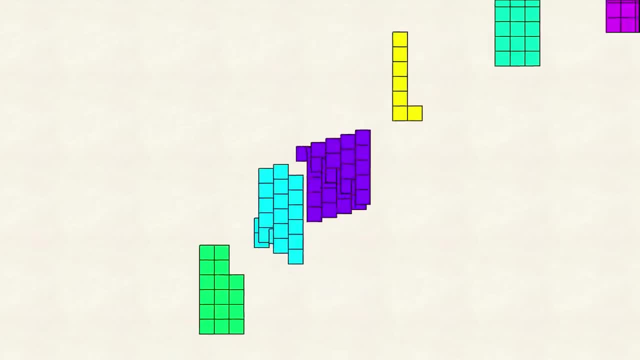 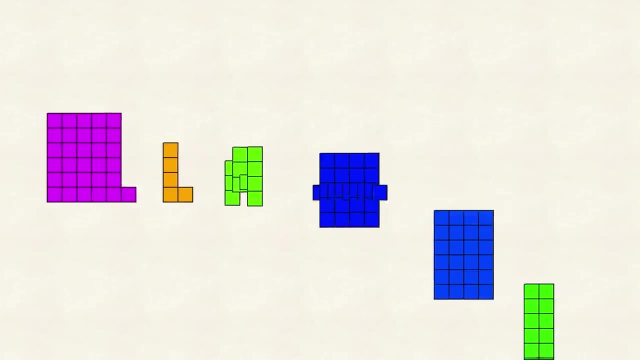 where current problems are and then thinking about ways to circumvent them. It was those little insights that got us closer and closer to the complete proof. Even though the actual formulas for extending ninja pairs did come from a computer and are quite impossible to find by hand, they were not what made our approach work. 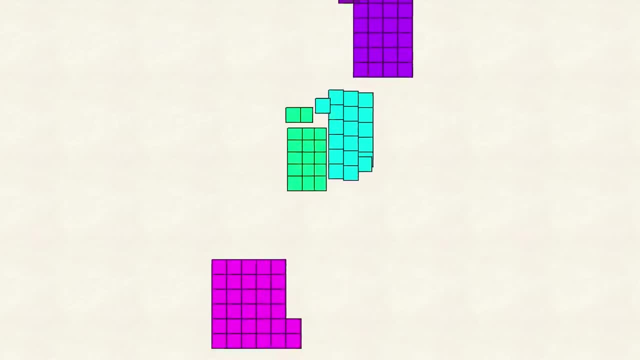 It was our reasoning that helped us to understand what rules or formulas we need. The computer simply did the dirty work By crunching the numbers And actually finding them.